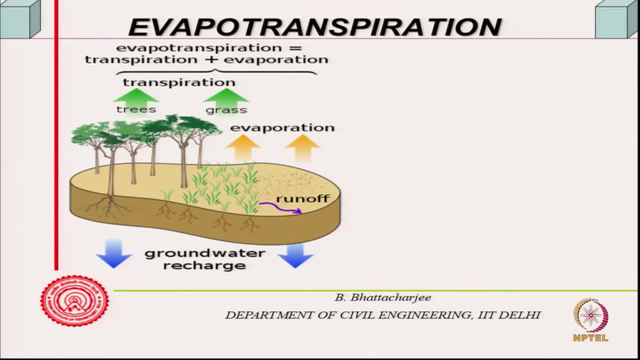 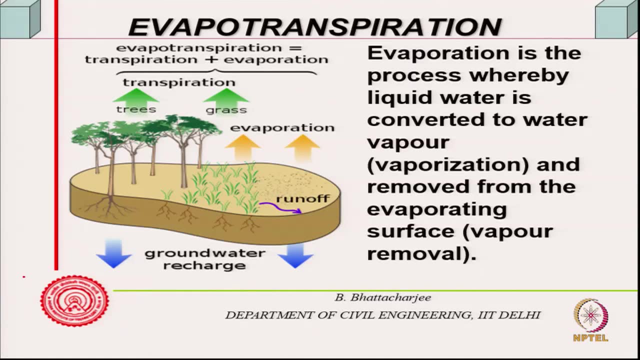 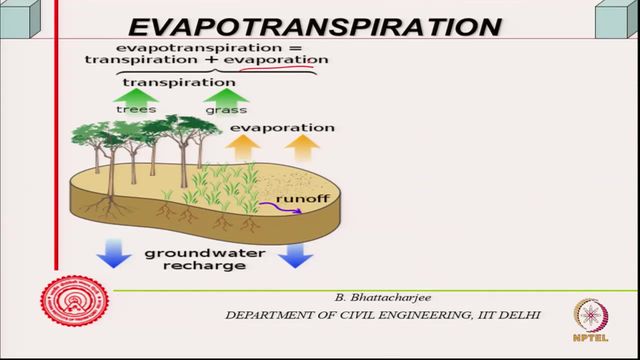 how does it change the microclimatic features such as humidity or temperature? that is what we are looking into. So two things happens with trees, actually the transpiration and evaporation. So trees, basically there will be evaporation from the trees and transpiration, So we call. 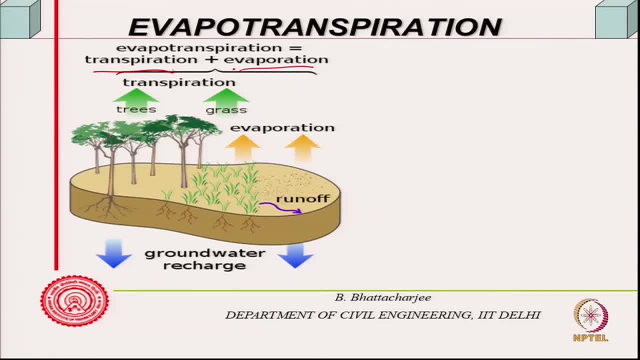 it evapotranspiration. this process is called evapotranspiration, So evaporation takes place from the surrounding ground- you know surrounding ground- and there is a transpiration from the green trees itself. both together- you know both together- or there will be evaporation. 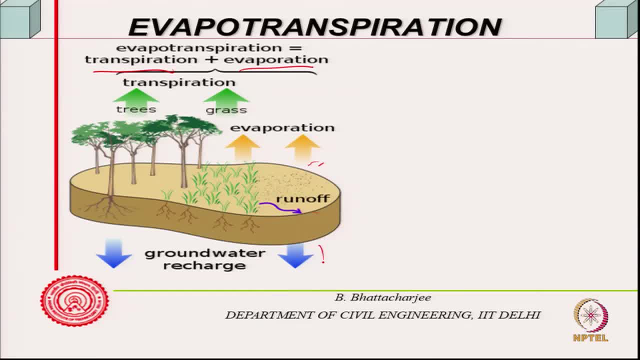 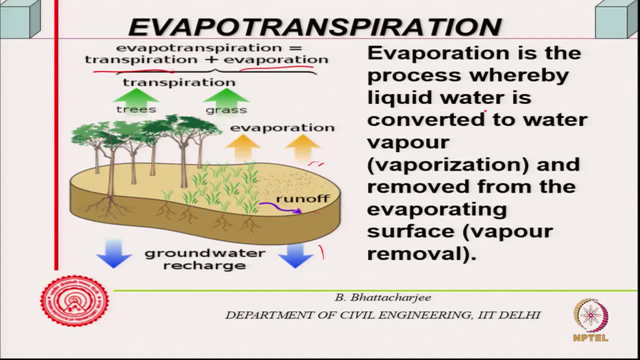 from the green surfaces as well, And there will be some runoff. some goes to the ground water, some goes to the ground water, right? So evaporation is a process whereby liquid water is converted to water vapor and removed from the evaporating surface, which could be ground as well as the plant. 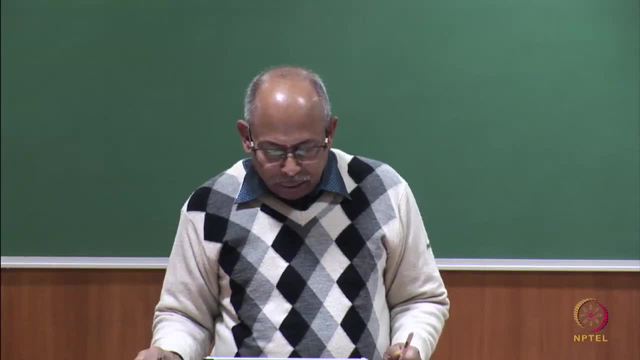 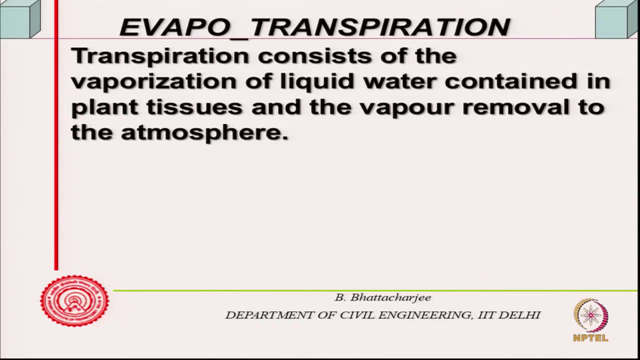 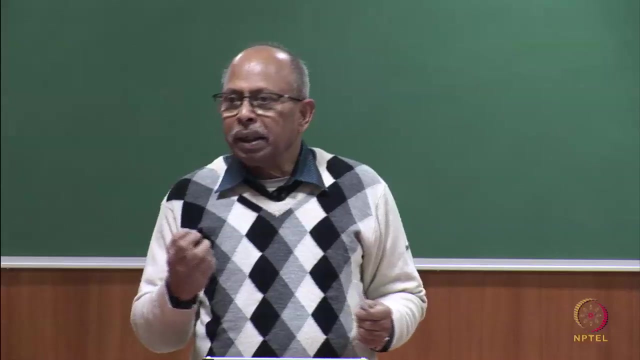 surfaces right. So transpiration consists of vaporization of liquid water contained in the plant tissues right And the vapor removal to the atmosphere. So in the process, in the biological process, there are water, evaporation takes place from the plant and you know you need water for. 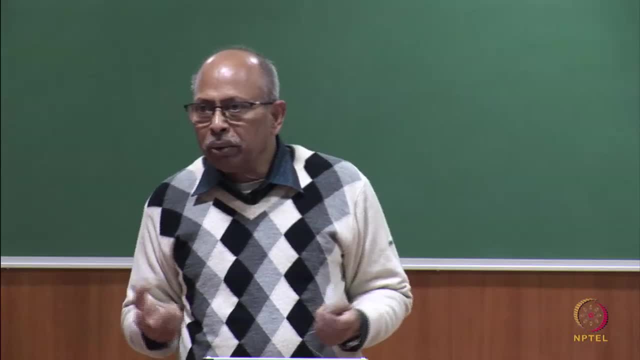 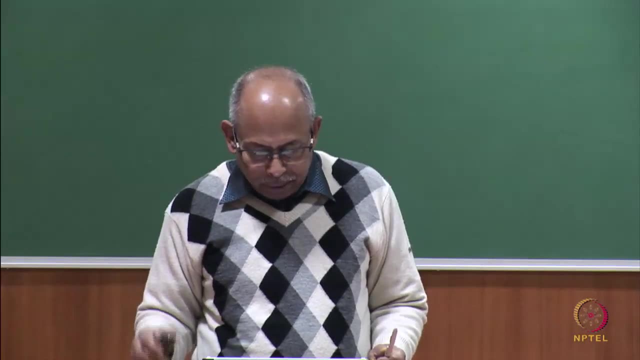 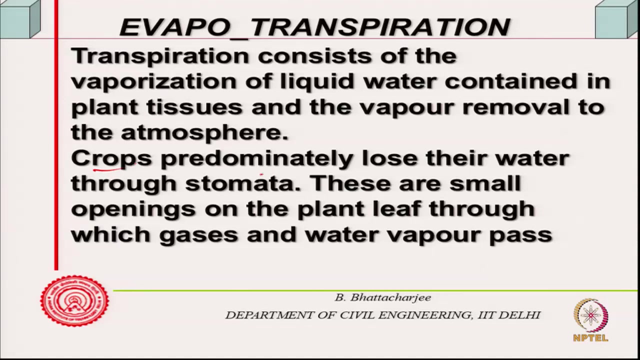 plant survival right. It is nutrients it picks up, and this from the plant tissue. there is water evaporation that takes place So that we call as transpiration. So these crops, or if we say trees, even Transpiration- predominantly lose their water through what we call stomata. These are small. 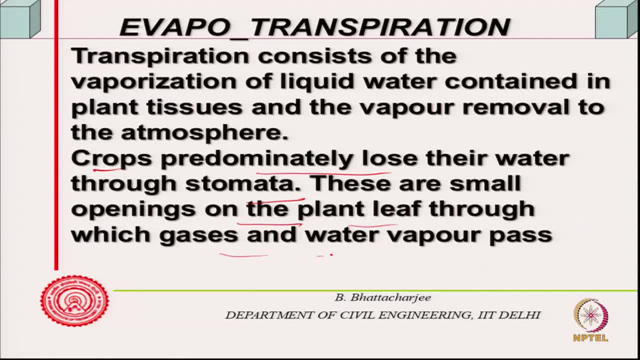 openings in the plant leaf through which gases and water vapor pass. So there is evaporation from the plant, also because the water is needed for carrying the nutrients right, and then water is also evaporated out from the plant surfaces. So the combination of these two. 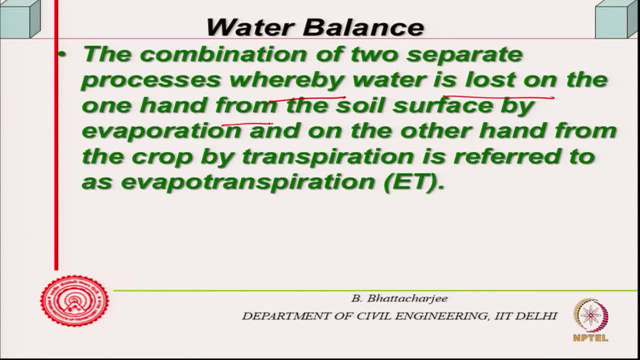 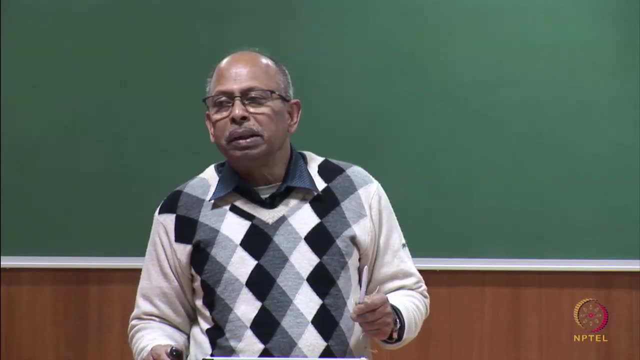 separate processes. So the process whereby water is lost, on one hand, from the soil surface by evaporation and, on the other hand, from the crop of by transpiration, is referred as evapotranspiration. So obviously, what will be its effect? It will tend to increase the relative humidity locally. 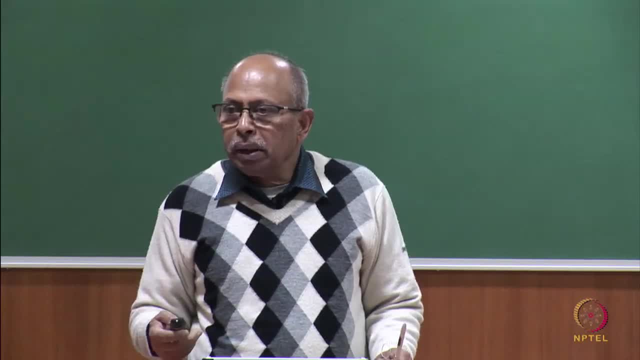 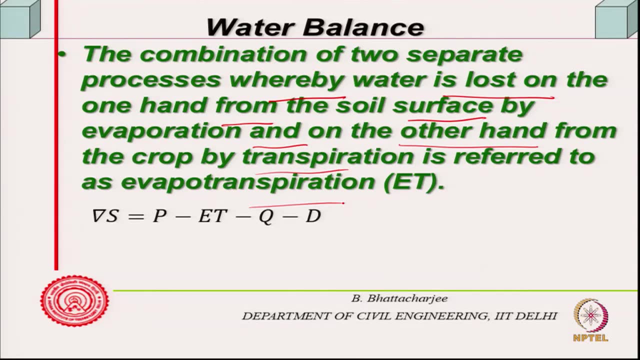 and since the evaporation is occurring, it would reduce down the temperature. it will reduce down the temperature, right? So evaporation, So evaporation, So evaporation is what it means. This is so we can write it like this: Delta S is the. 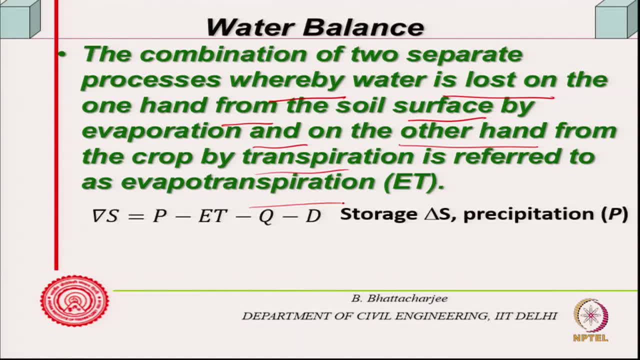 storage. you know, P is the precipitation, the rain or whatever it is, and Q is the stream flow, runoff, and then ground water recharge is D. So this is what it is. So evapotranspiration is this part. So this is what it is now. So this is what it is right. So evapotranspiration is this. 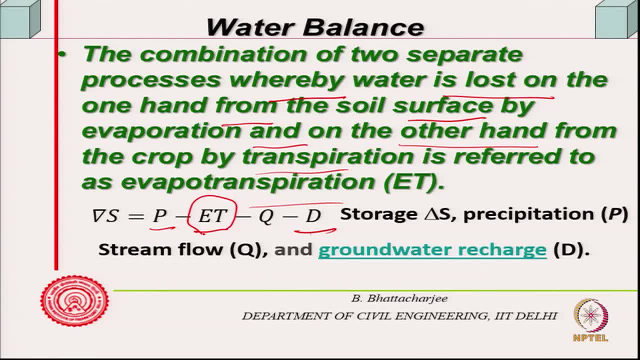 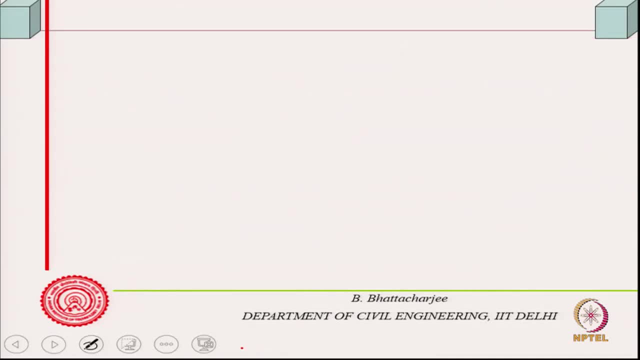 through which water is lost to the atmosphere, but then it does cooling, while this Q is actually not really much useful in the sense that it straight away runs off. So it does not take part in anything else and delta S will be the storage in the ground. 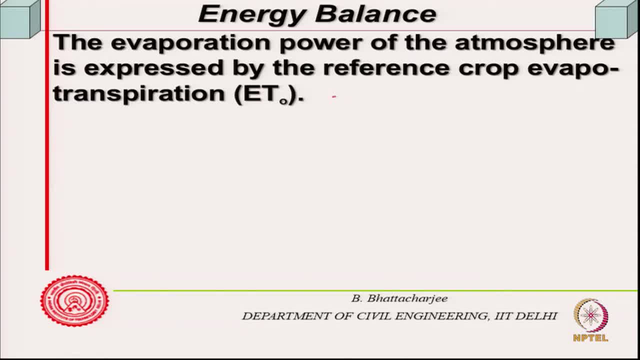 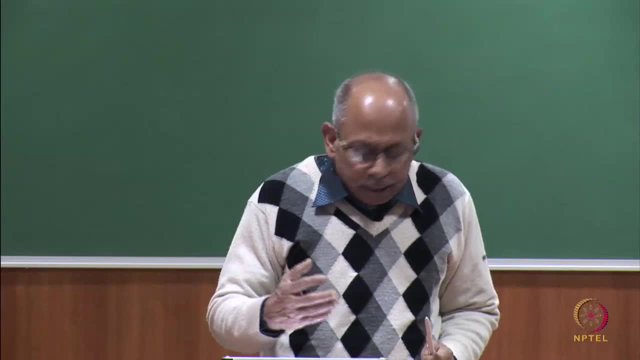 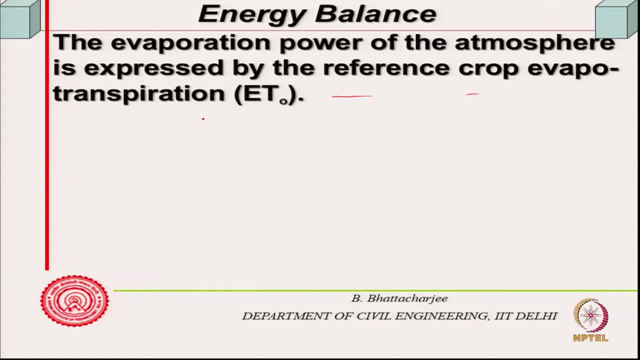 water system. So evaporation power of the atmosphere is expressed by what is called reference, crop evaporation, evapotranspiration. Now this has been modeled So you can actually model this process for agricultural engineers. actually they have done it actually. So they take a crop preference, you know crop evapotranspiration. 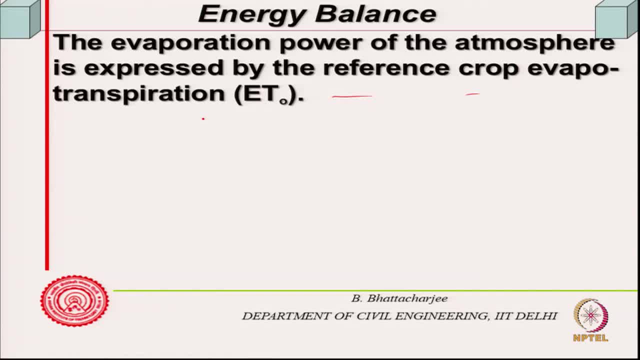 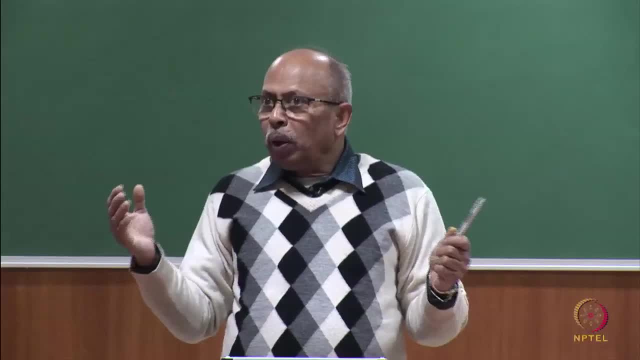 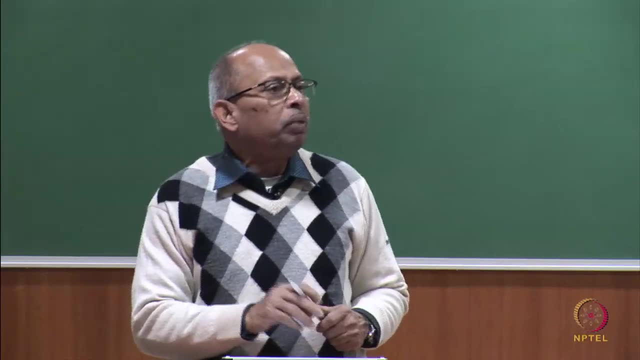 As we shall see this, this model, if you can apply, for example, you can actually compute, as we shall see, What is the likely relative humidity change. It will change because of the green trees around this place. The example I will have is of Humayun stone, where there are plenty of trees around the 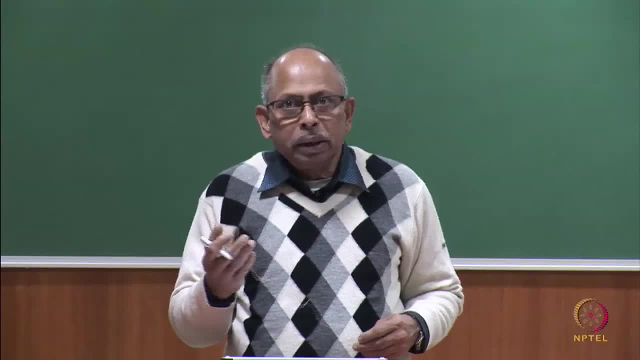 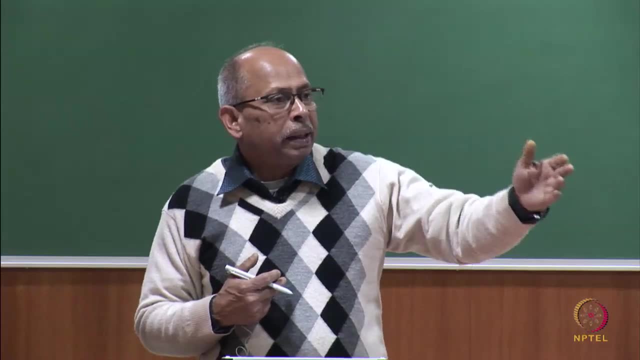 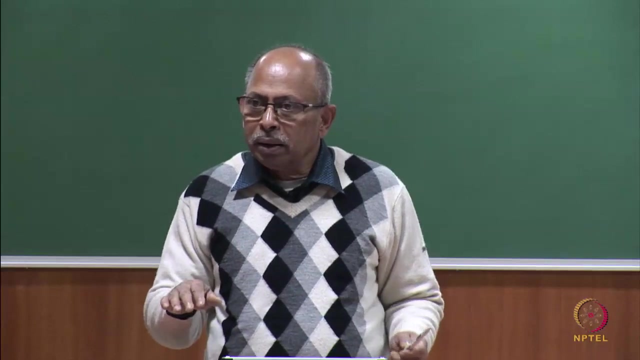 monument and it showed that there is a reduction in the temperature compared to measured temperature. in one of the station- atmospheric station like South Dajang airport, which is not very far off, Measured temperature is lower, But measured relative humidity is lower. So this is what you can see. 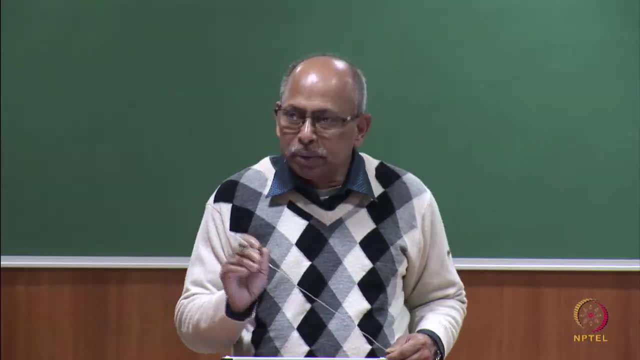 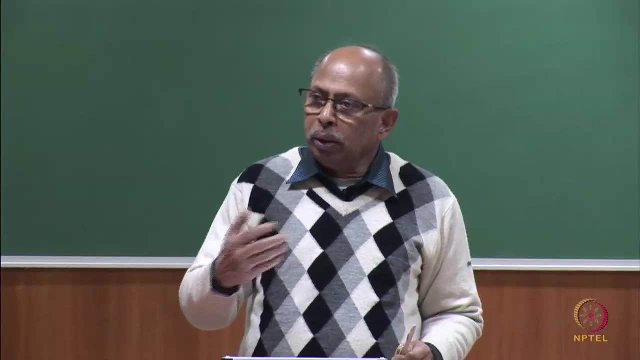 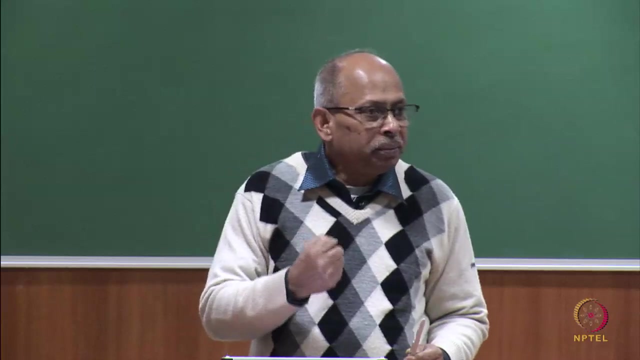 Higher relative humidity is higher. So this is the whole purpose. Purpose is to see what is the basically the physics or physical mechanism behind this kind of thing, So that you can actually look into any other place as you want. Now, agricultural engineers have actually used this kind of concept before for the purpose. 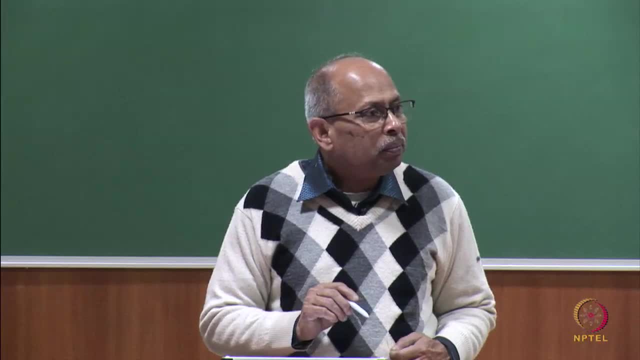 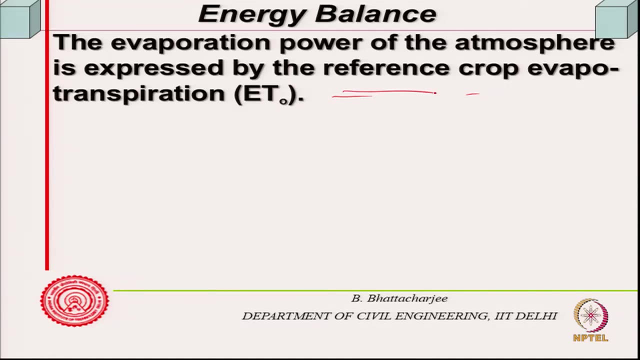 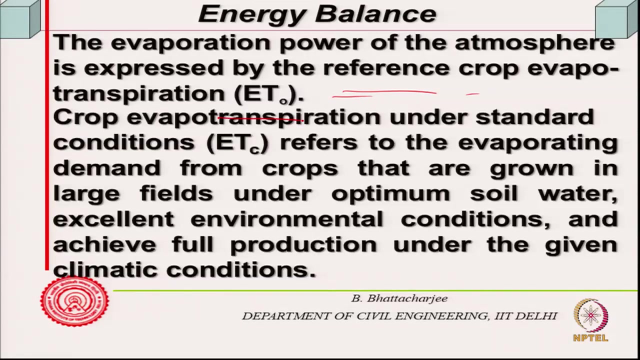 of crops, So the idea is borrowed from crop, So crop evapotranspiration. So they define something called standard or reference crop evapotranspiration Or reference crop condition for which the standard evapotranspiration is ET0.. Now crop evapotranspiration under standard condition refers to the evaporating demand. 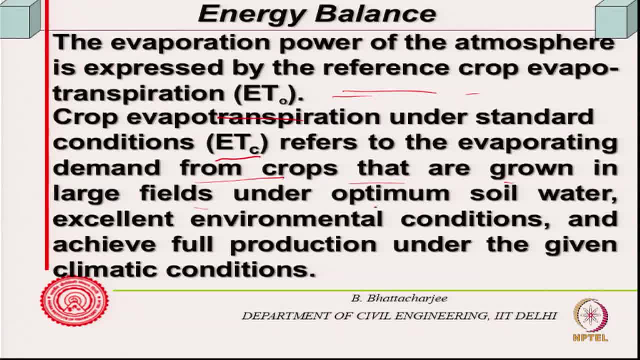 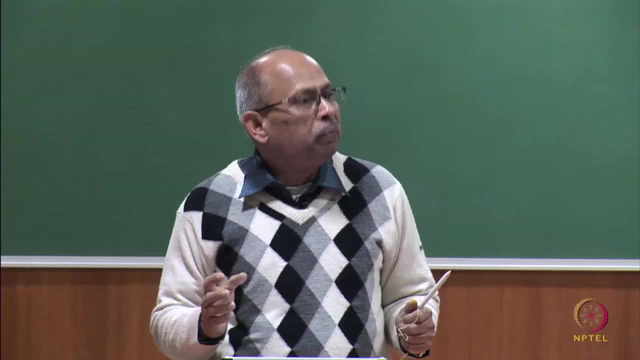 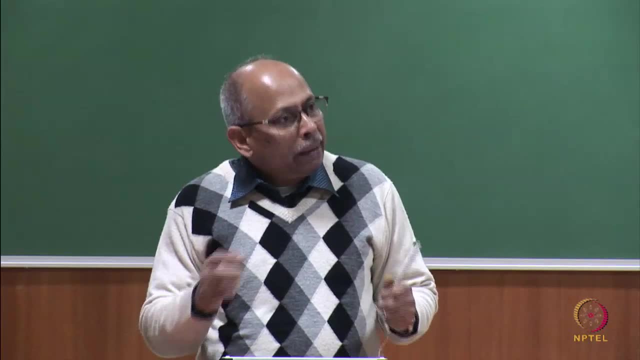 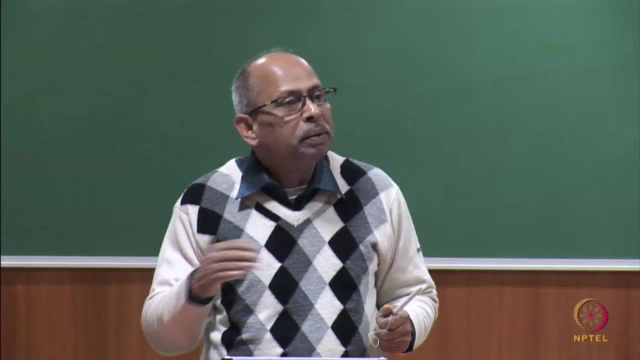 from crop that are grown in large field under optimum soil, water condition and excellent environmental condition, So and achieve full production under the given climatic condition. So basically, So for most conducive condition, for standard crop, this has been established, And then for any other crop and any other condition, you have some multiplying factors. 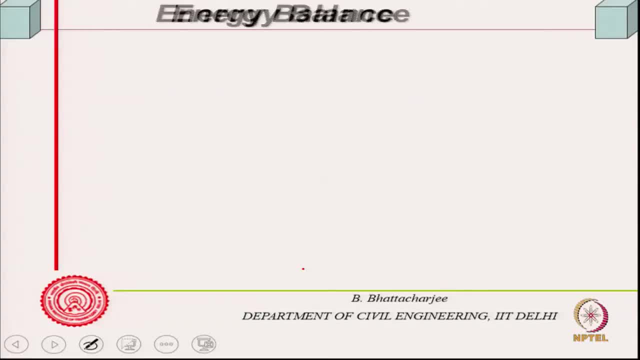 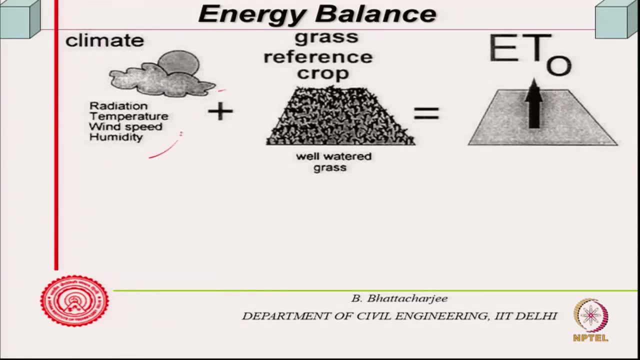 to find out the amount of evaporation, say millimetre per day or whatever it is. So if you look at first, you know both energy balance as well as the. so basically, this is the precipitation radius. So this is the precipitation radius. So this is the precipitation temperature with humidity. 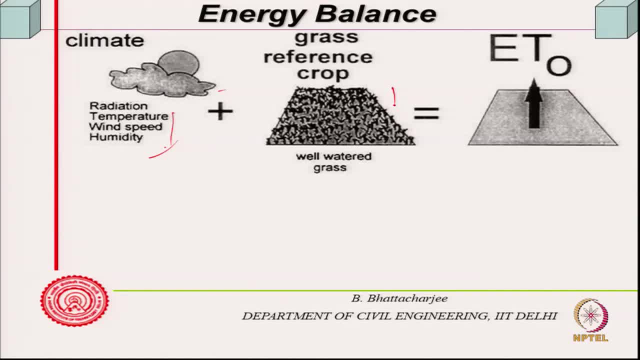 Now, reference crop is a specific type of crop with a given height and leaf condition, which is well watered grass, as you should see. you know, And later on, 12. it is actually 12 centimetre high and that is what we call as standard. 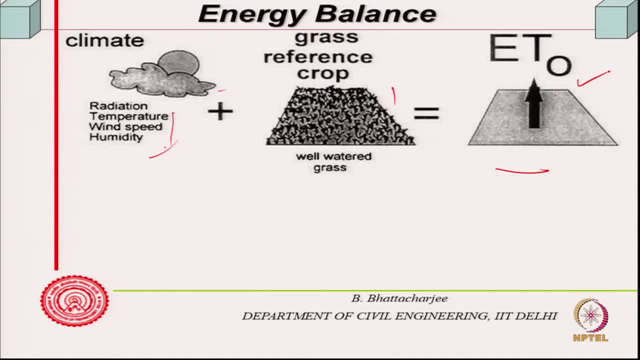 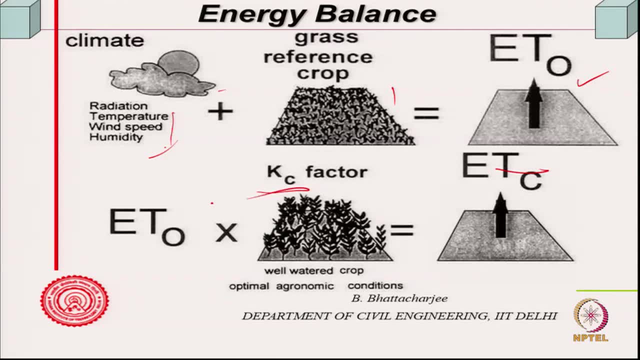 condition under which we define as evapotranspiration 0, I mean, you know, subscript, So basically the standard. This is multiplied by a factor. So ET0 multiplied by a factor for well watered other crop, not the grass, then you get ETc. 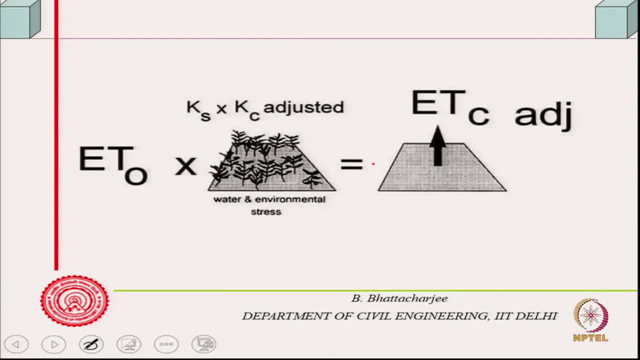 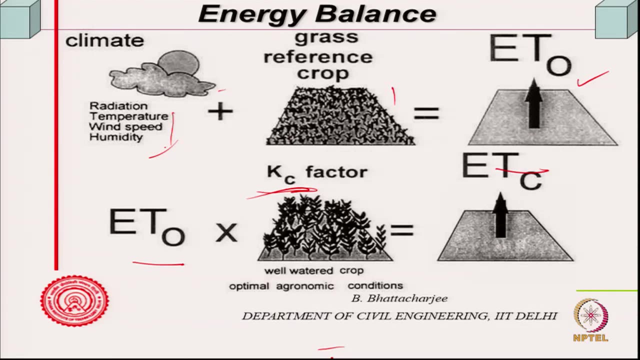 So that is the standard one, in fact, for type given type of crop. And then if water and environmental stress is there, that means water is not optimal or right kind of you know well watered optimal, you know agronomic condition. if it is not that, then you multiply by another factor. 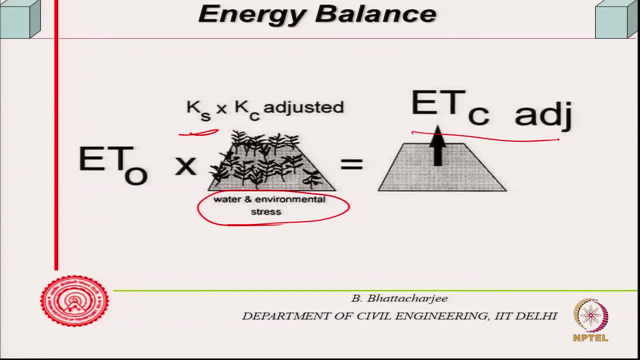 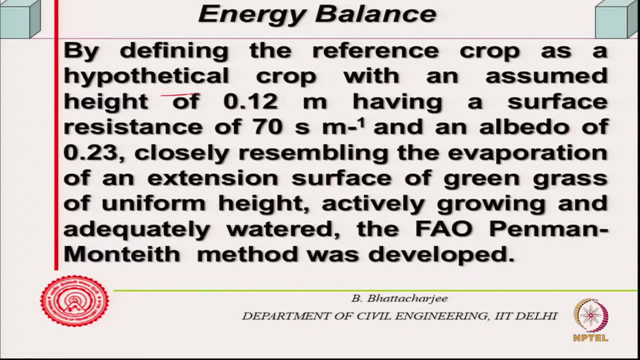 So this is ETc adjusted. you know that is how it is done. So for you know, for crop this is done right. So by defining the reference crop as a hypothetical crop with an assumed height of 0.12 metre, that means 12 centimetre. 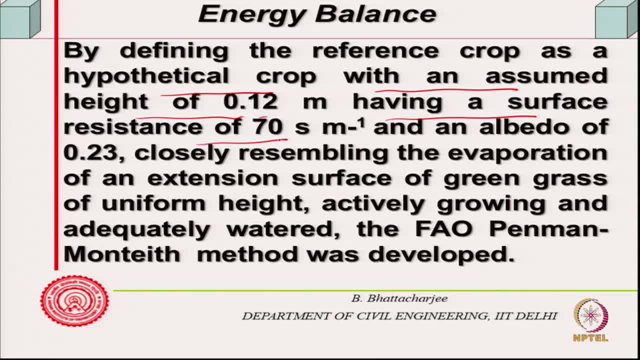 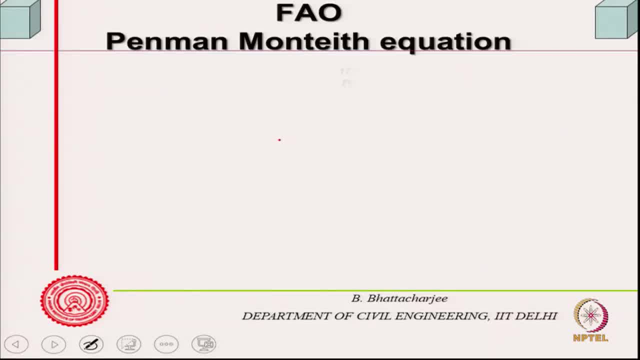 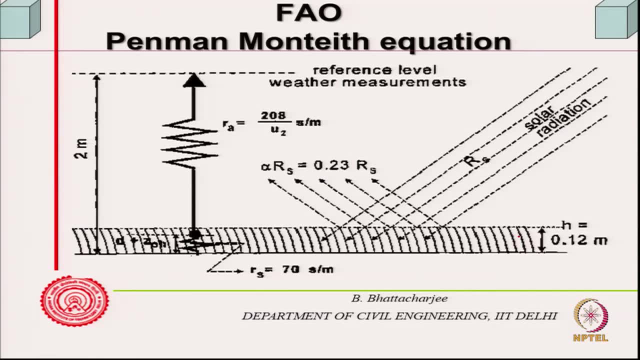 Right- 12 centimetre- And having a surface resistance. now, I think I will come to this statement later on. let us look at this diagram. let us look at this diagram, something like this: I have this height of the crop grass: 12 centimetre. solar radiation falls on to it and this is 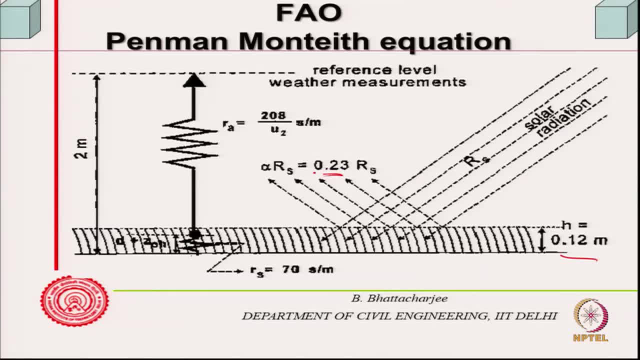 the albedo Part of it goes out, you know. So this is what is: falling: solar radiation falling on to it. Now there is evaporation occurring from here. So there is a resistance offered. there is a resistance offered which is in 1 over velocity. 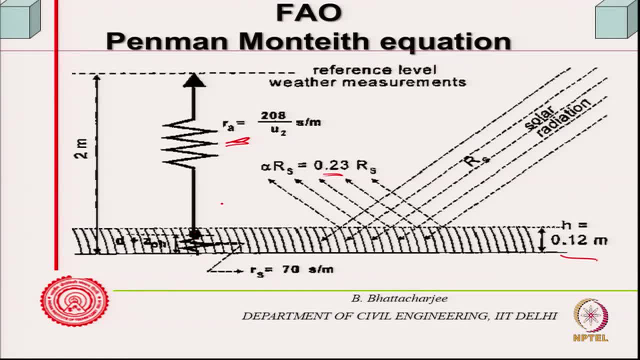 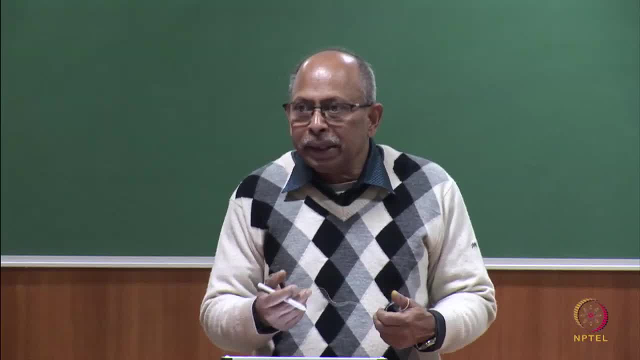 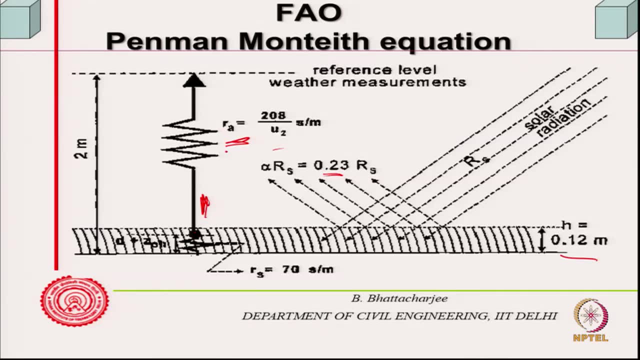 term. So velocity is metre cube per metre square. Velocity is nothing but flow per unit area, right. So 1 over that flow is a resistance. that is what we are talking of. So there is a resistance offered here, Right, And this resistance to this evaporation, because it is a flowing vapour, is flowing. 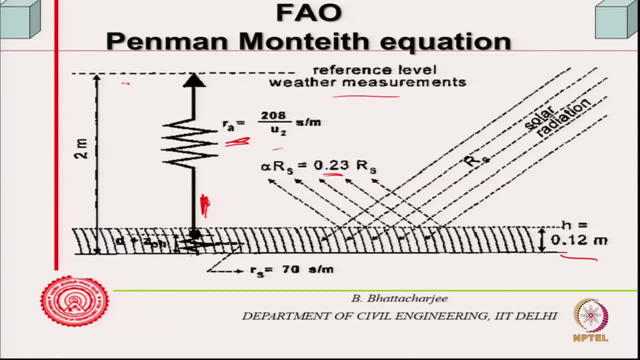 So what reference level? weather measurement is done at 2 metre height. So temperature, relative humidity, etcetera, measured at 2 metre height for 12 centimetre or 0.12 metre crop, and there is one resistance here as well, which is assumed to be 70 second. 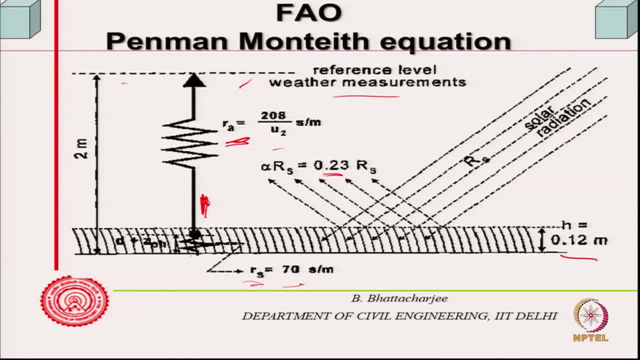 per metre Right. So this is 1 over velocity. So this is, you know this from experiment, empirical observation. they would have found out. and this resistance from here to there is actually resistance of the air. This is resistance of the crop itself and this is given as 208 divided by velocity, where 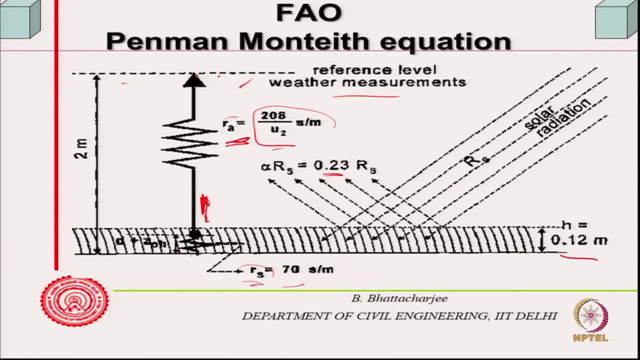 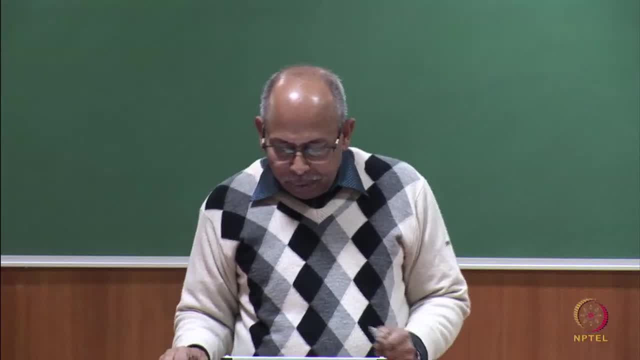 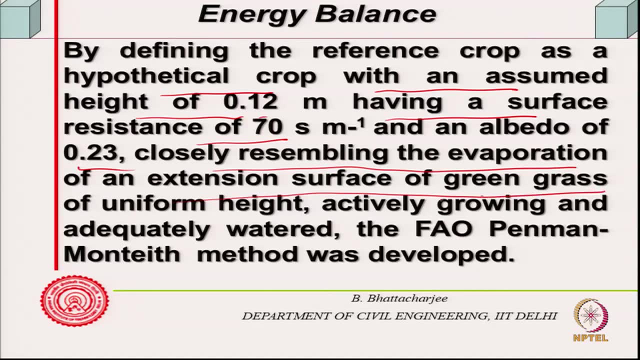 air velocity. If the air velocity here is high, obviously more evaporation would occur. resistance will be less. So that is how it is done, And albedo is taken as 0.23, closely resembling the evaporation of an extension surface of green grass of uniform height, actively growing and adequately watered. 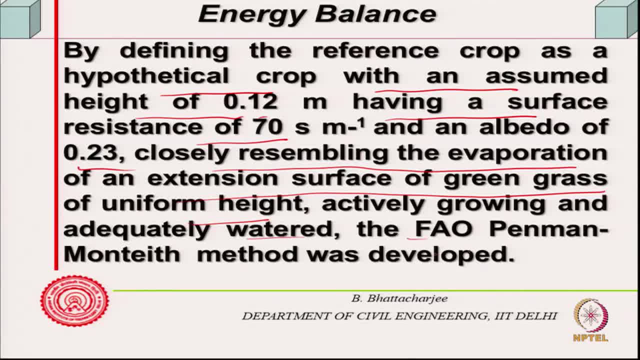 The you know, FAO Penman-Monteith method is developed based on this actually. So this model- Right, Okay, Federal Agricultural Organisation, because it is US American Society of Civil Engineers, they did it, So this model was developed based on this model was developed based on this for reference. 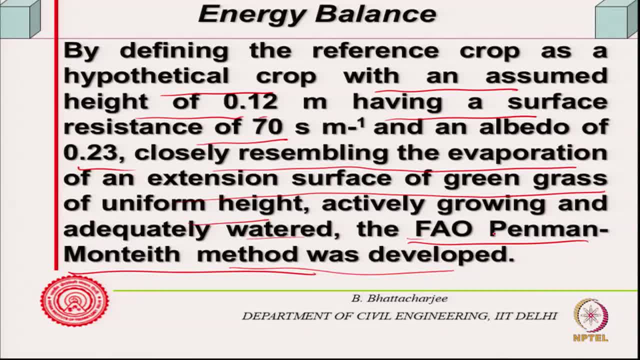 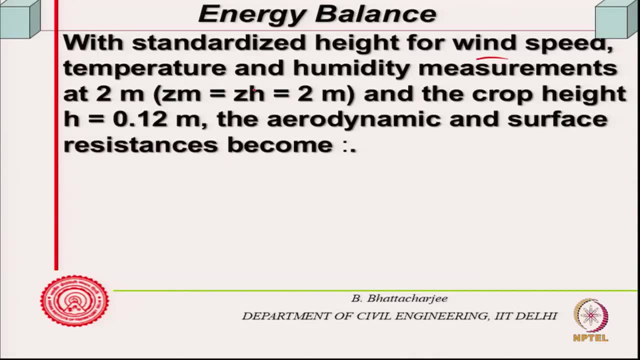 crop with measured, you know, accepted- resistance value from the soil to the crop and resistance value from crop to the 2 metre standard height, Right? So this is what it is. So standardised height for wind speed, Temperature and humidity at 2 metre and crop height. of this, the aerodynamic and surface. 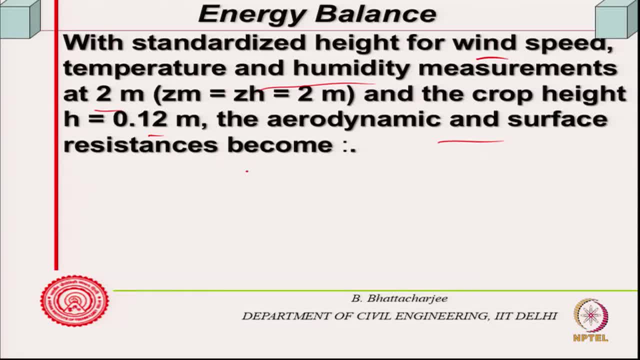 resistance has become. So first is the surface resistance, another is aerodynamic resistance, So RS and so RA is taken as 208 by U2, as shown in the diagram, and the UT is the wind speed at 2 metre height, and RS is 70.. 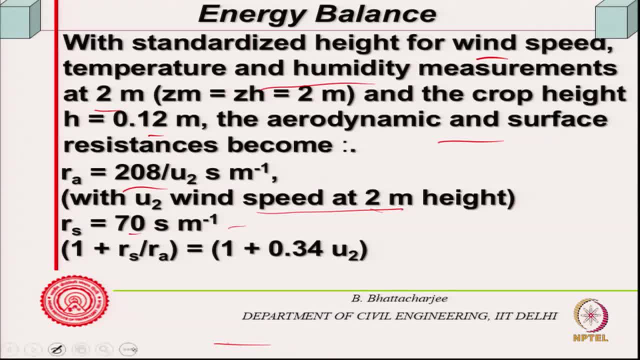 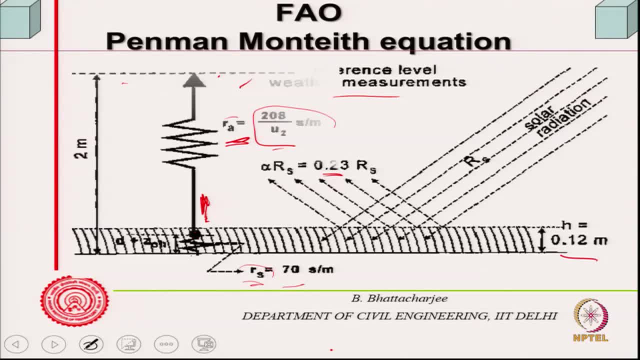 So this ratio is useful somewhere. We shall see that resistance, you know, 1 divided by 1, plus resistance of these two. So this is, this is Penman-Monteith model. actually this is the Penman-Monteith model. So this model can give you the evapotranspiration under standard condition. 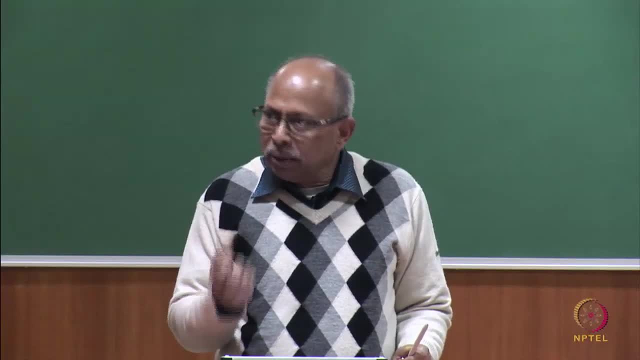 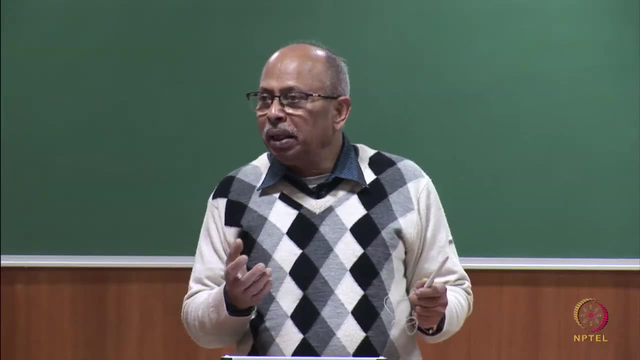 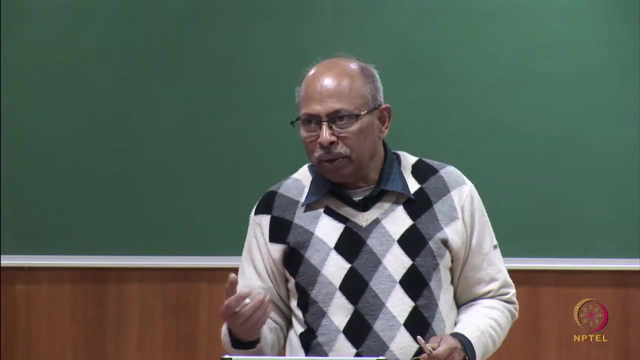 Right, It can give you, under standard condition and once you know the standard condition for your type of crop, which is also- they have listed down For what sort of crop- What should be the factor K, and then you can apply that and find out. 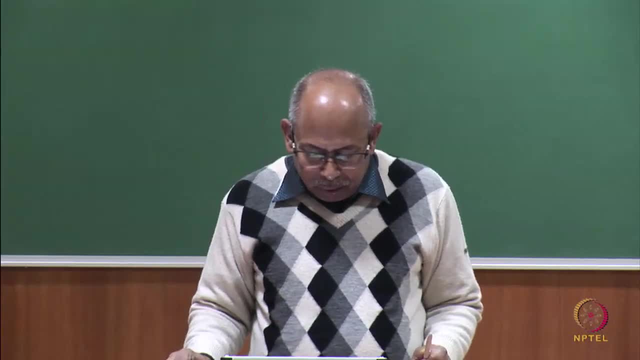 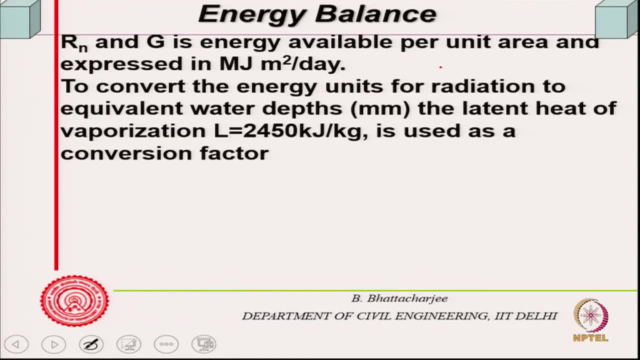 Right, Okay, So this is the basic principle, So right, so this is what I said, and Rn, that is the normal radiation. we are using Rn. here, the I mean they are using Rn. the notation I have kept it: Rn is the normal radiation. 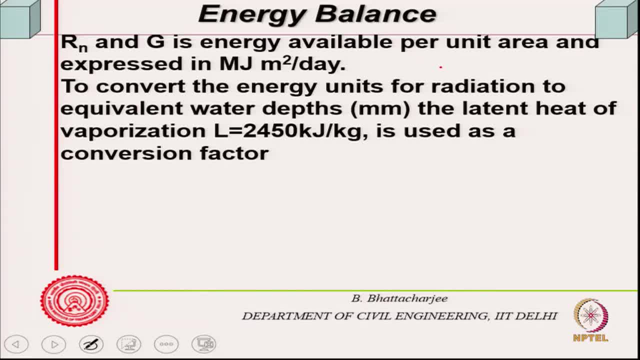 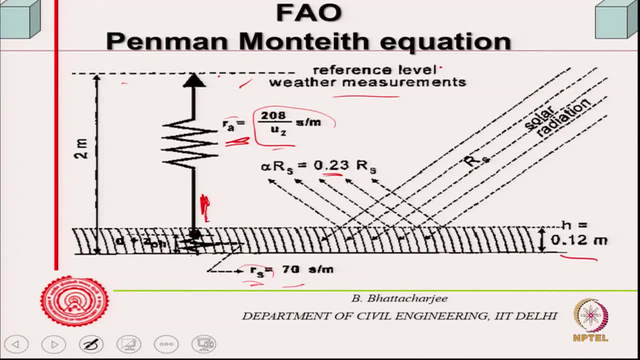 Okay, G is the energy available per unit area and all these are expressed in mega joules per metre square per day, you know. So if you look at it in this diagram, this is the normal radiation. supposing I am calling it Rn here, of course it is shown as S, as a solar radiation. 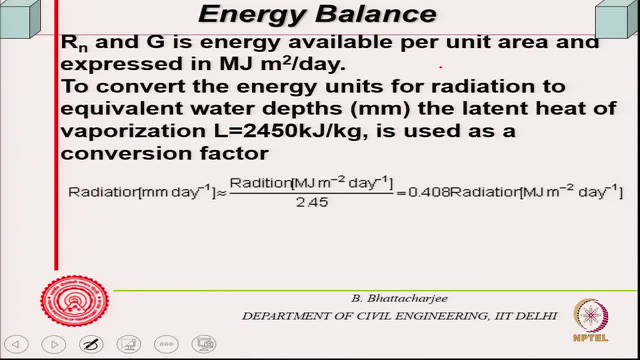 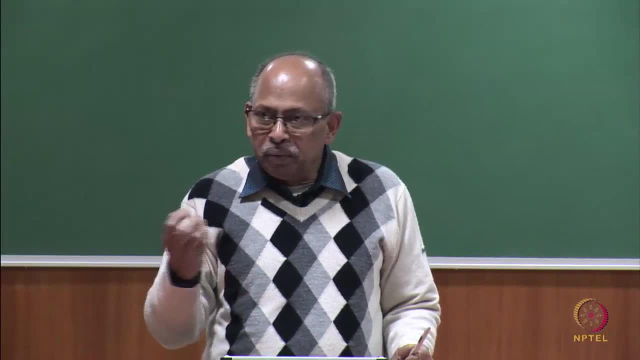 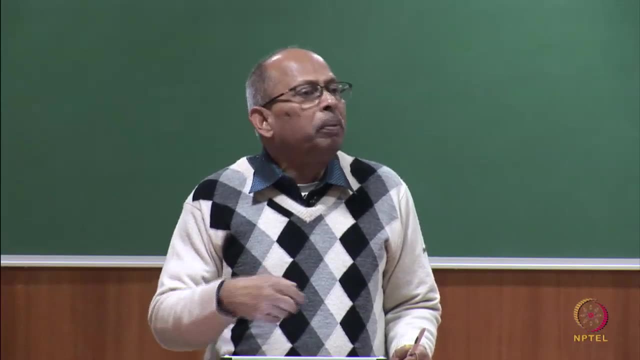 So this and G is the energy available per unit, because some of this radiation will be reflected back, Some will be available. Okay, So this is occurring. energy must come, latent heat of evaporation must come. So if radiation is known to us, some of this energy will be actually absorbed for evaporation. 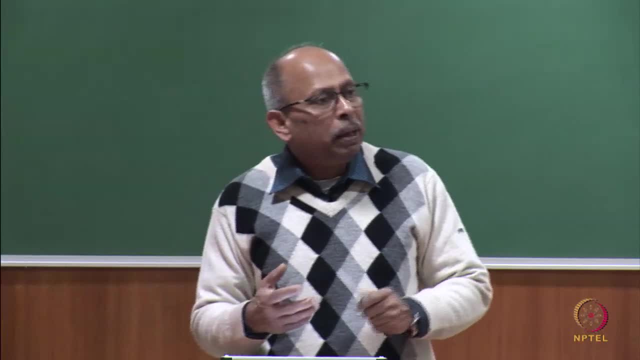 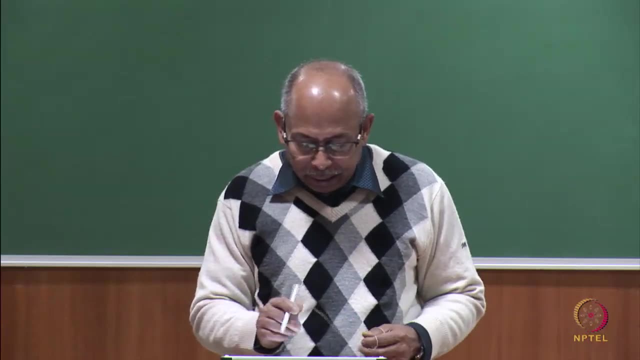 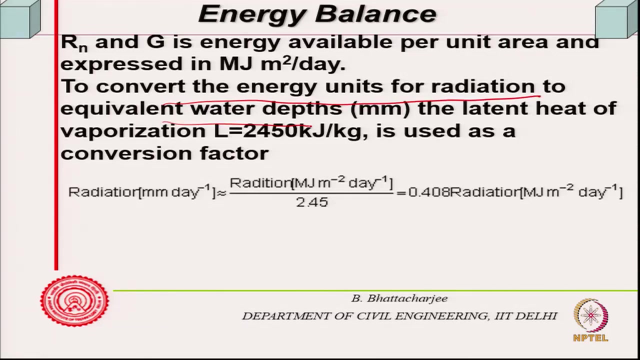 purpose, will be consumed in evaporation purpose and some will be, you know, some will be reflected back and, you know, will go on heating and things like that. So to convert the energy units for radiation equivalent to water depth, so you want to find out how much is the water depth, right? 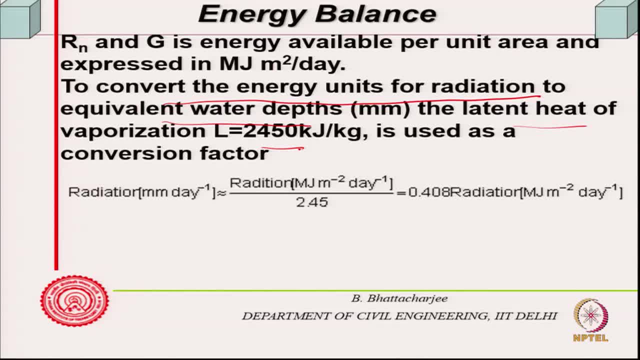 The latent heat of evaporation taken as 2450 kilo joules per kg, So radiation corresponding to radiation in mega joules per metre square per day. I want to find out how much is the evaporation corresponding to the radiation in millimetre per day, because 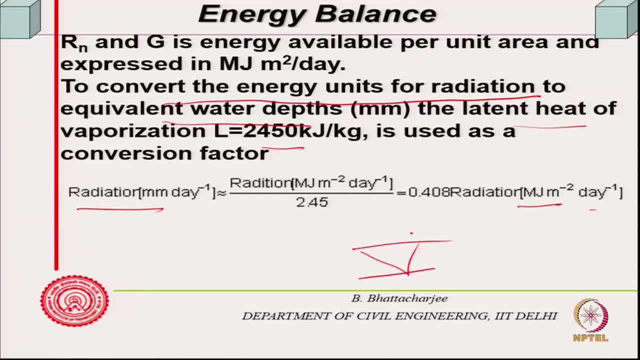 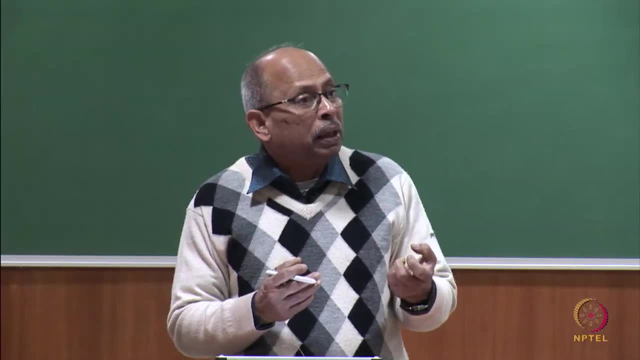 it will be evaporating from the some depth Right. So radiation mega joules per day divided by 2450 latent heat of evaporation. So if I know the total energy coming in this divided by latent heat of evaporation will give me the quantum of water that can evaporate from the radiation received. quantum because 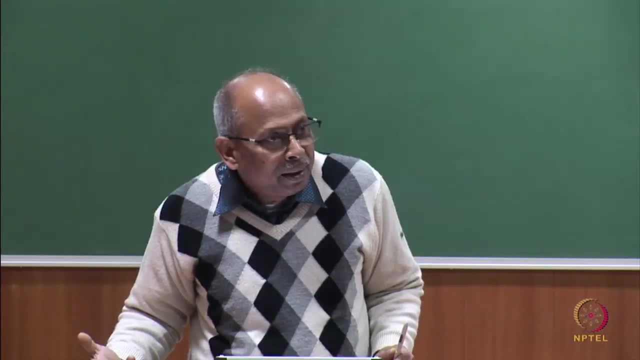 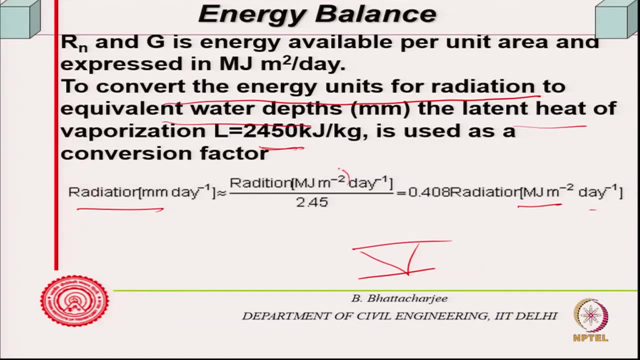 after all, if the evaporation is to occur, the sunlight is also needed. You know the energy is needed in order that evaporation takes place, Right So? So if mega joule per metre square per day is the amount of radiation, this divided by 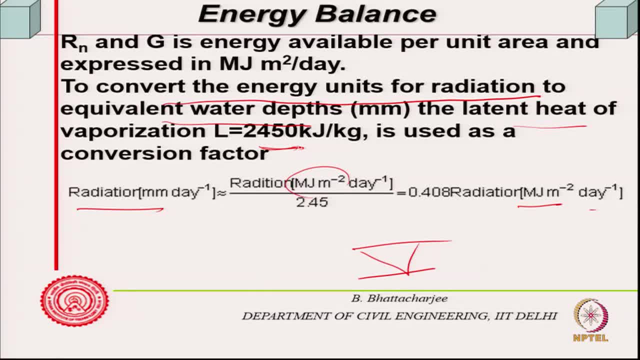 2450, 2450. this is in kilo joules per kg divided by 1000 will be. this is how it is, you know. So this divide, this is mega joules. I multiply by 10 to the power 3, I get kilo joules and 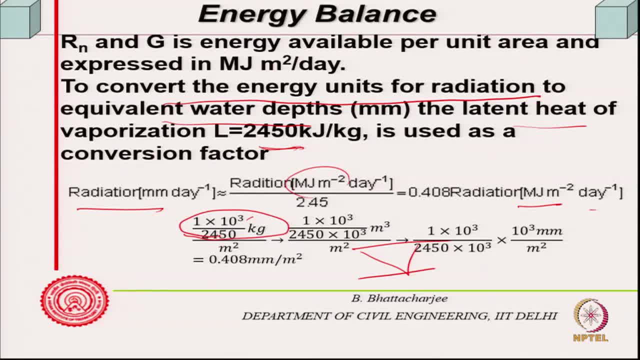 this is 2450.. So that much kg of water will be Right. So this will be this multiplying factor I am trying to find out. I am trying to find out a multiplying factor, this value multiplied by the radiation. So whatever radiation I get, multiplied by factor, that is what will give me millimetre. 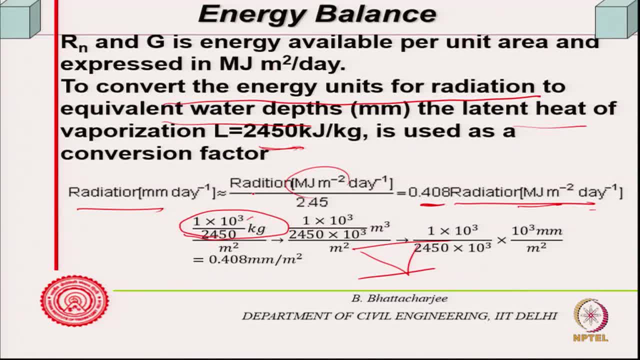 per per day. So radiation is. this is in mega joules per metre square per day. multiplied by 1000, divided by 2450, that much kg of water or moisture will evaporate. this, multiplied by for 1 unit mega joule per metre square per day. 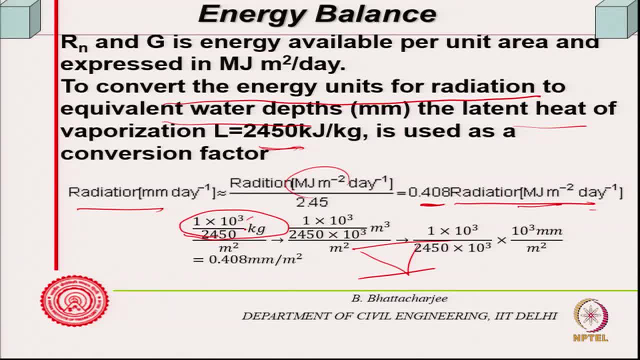 For unit mega joule per metre square per day. this much kg of moisture will evaporate right, So per metre square anyway, this is per metre square. so mega joule, so kg per metre square, will come per day. Now this, multiplied by 10 to the power 3, because I want to convert this metre into this- is: 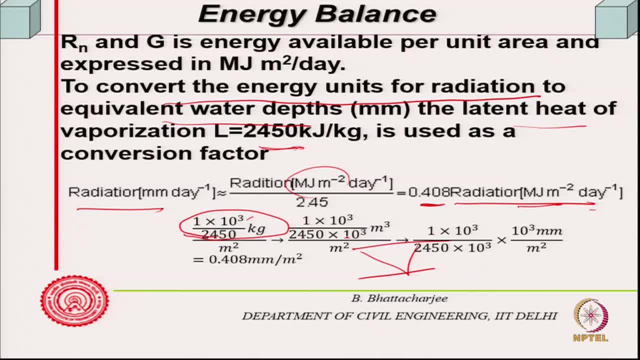 this will be in kg. kg divided by metre 1000 will give me in metre cube, because density of water is 1000 kg per metre cube, Right, So meter depth of water that would be actually evaporating for the amount of radiation that. 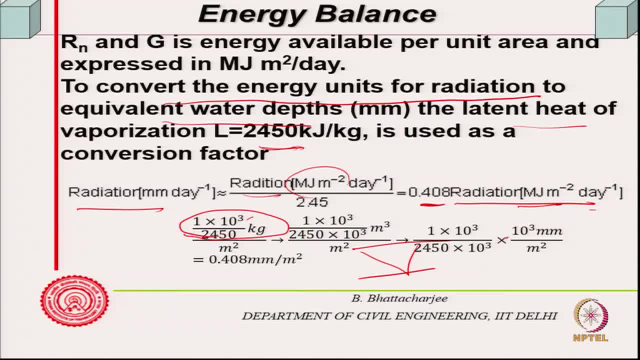 is coming in per unit radiation. Now this if I get, I get something like this: 10 to the power 3, you know. so, millimetre, if I want to convert, I will multiply this factor by 10 to the power 3.. So I get 1 by 2.45, which is 0.408 millimetre square per metre square. 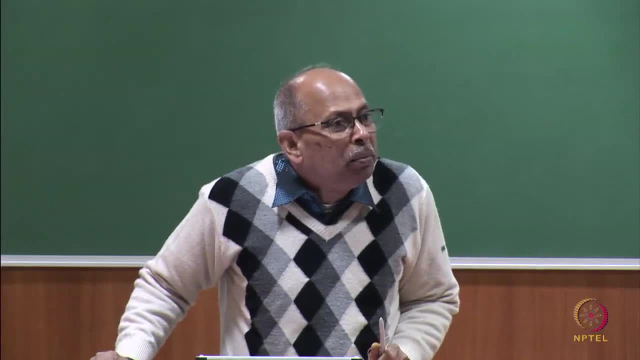 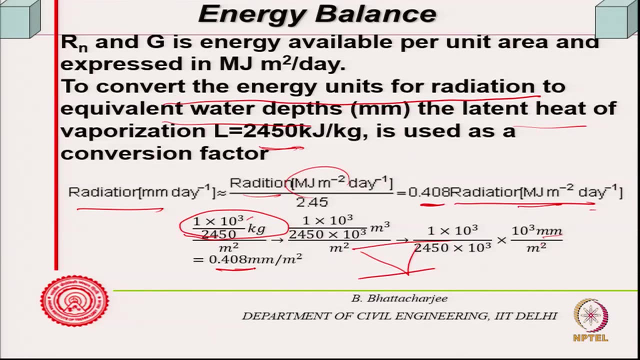 So for unit radiation unit, mega joules per metre square per day, The amount of water which will evaporate is 0.408 thickness. if it is fully saturated, if it is fully saturated, 0.408.. Now this comes into the equation. actually, this comes into equation. you see, this is 408. 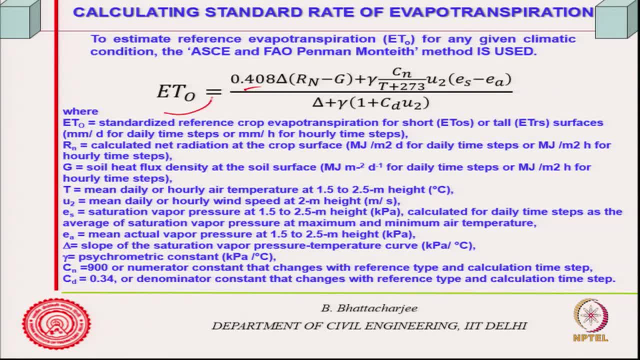 now it has got 2 component. as you can see this equation, there is a standard, standardised reference crop evaporation. this is what they have developed, this equation. so this is this: Rn is the amount of radiation. The amount of radiation that is coming in, G is going out into the ground. 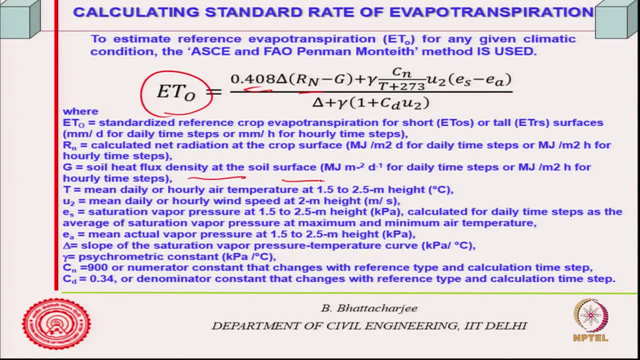 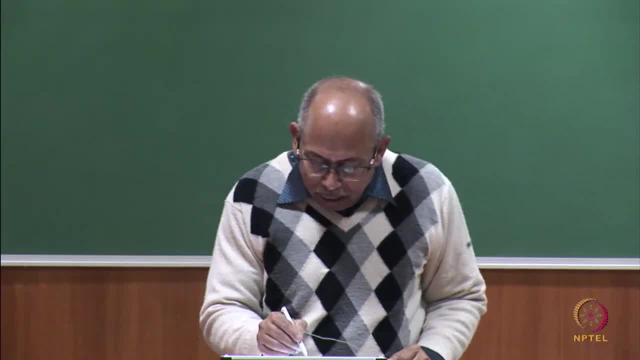 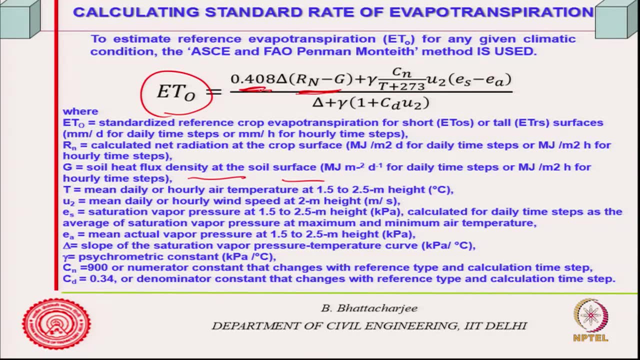 So G is the soil heat flux density. whatever is absorbed by the soil, Rn is the total coming out per unit area. a part of it will be absorbed by the soil. remaining radiation multiplied by 408 is a millimetre per day. But evaporation also requires, you know, vapour pressure difference. evaporation will occur. 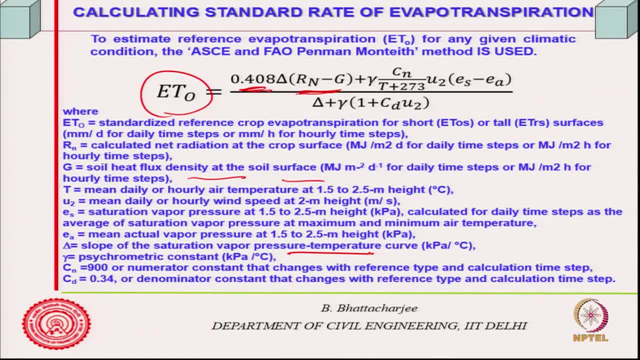 depending upon relative humidity Or vapour pressure difference, because if the vapour pressure difference is not there, evaporation cannot take place. is a fully saturated, So this is the slope of the saturation of vapour pressure, temperature right slope of the saturation, because moisture is saturated and there the evaporation is occurring at. 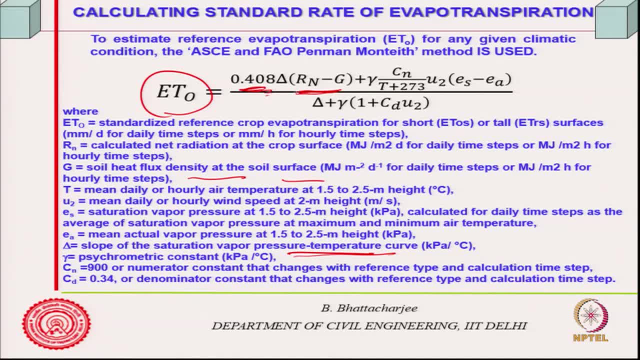 a given outside temperature. So this is, this gives me, this is this will be, you know, second part deals with velocity. second part deals with: So this is the evaporation that is occurring at the surface itself, at the plant surface itself, And this is related to the velocity somewhere above, if the due to depend upon the resistance. 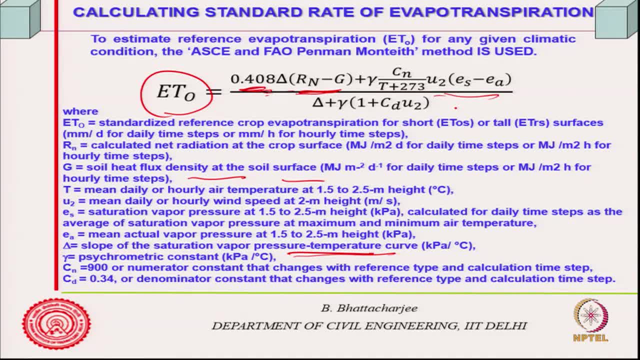 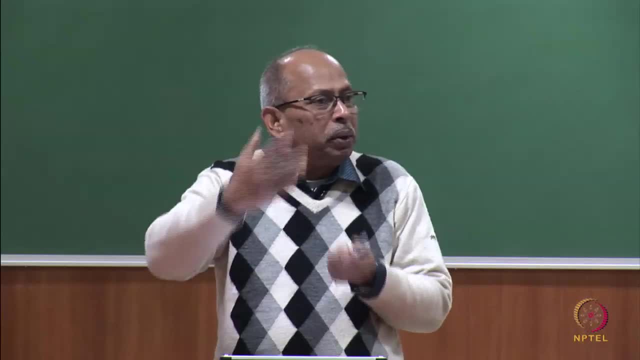 also the pressure difference between that point and the top surface. 2 meter at 2 meter. So Es and Ea saturation vapour pressure at 1.5 to 2 meter height, 2 meter height now I am considering. so first stage is at the surface itself evaporation. 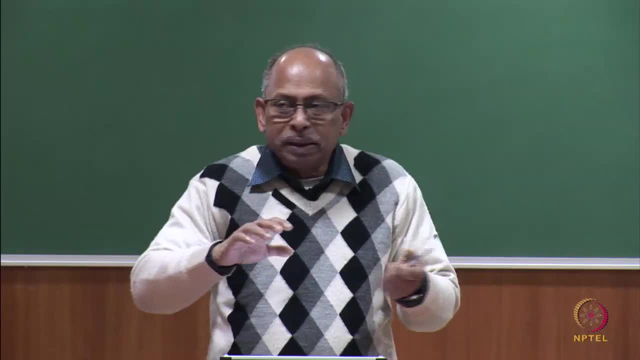 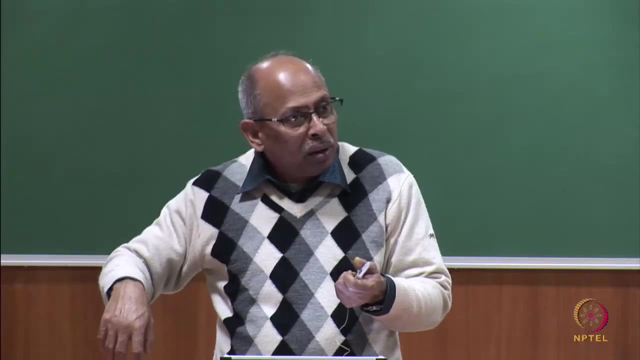 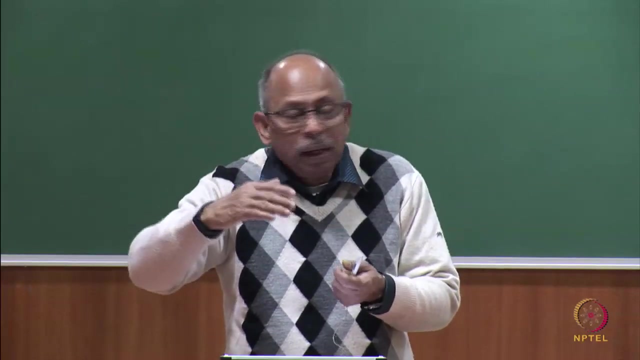 will occur centimeter thick moisture. I mean grass where the evaporation will occur. and that would occur because of the radiation coming in, minus the radiation that is going into the ground. that would cause evaporation. Second thing is: after that, also further evaporation will proceed from there to the 2 meter height. 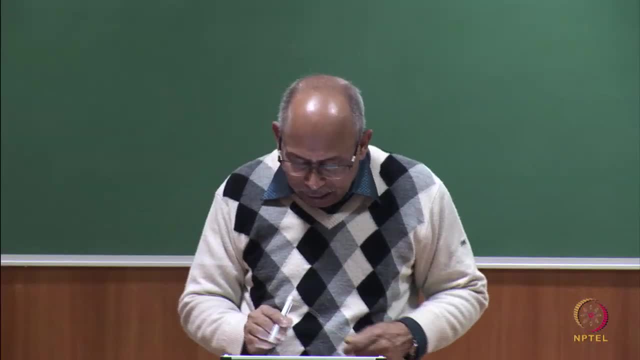 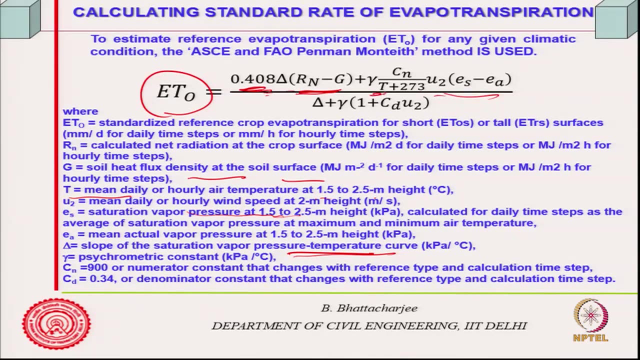 depending upon the relative humidity at the 2 meter height. So it is taken as 1.5 to 2 meter height. you know T mean temperature at T is coming, T would be coming here, that is an absolute term and gamma is again. the gamma is psychrometric. 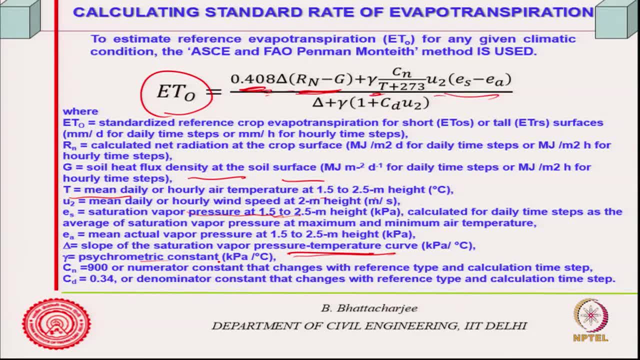 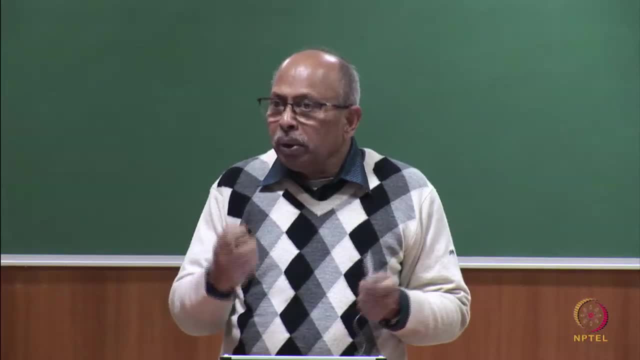 constant related to vapour pressure difference to moisture content. you know kPa pressure, I mean vapour pressure to per degree centigrade. So this is. I do not think I have talked about the psychrometric chart earlier in this course, but does not matter, we will not get into that details. but what we understand is in a psychrometric 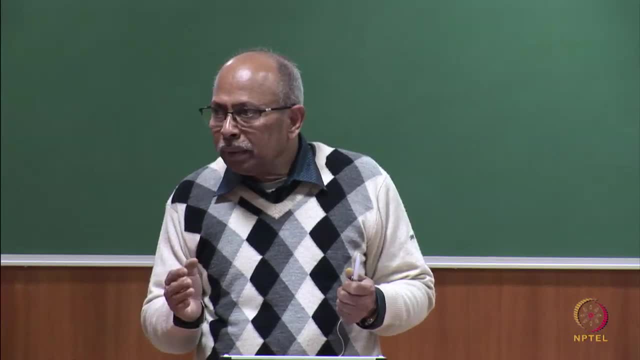 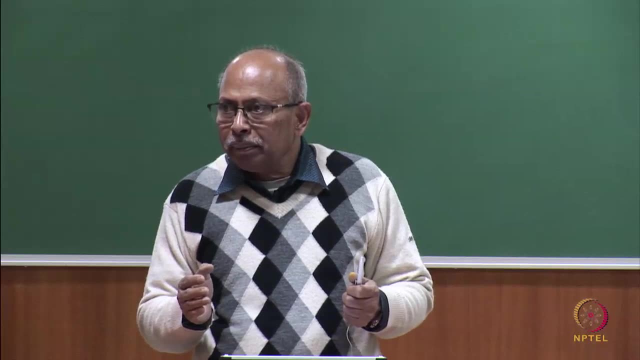 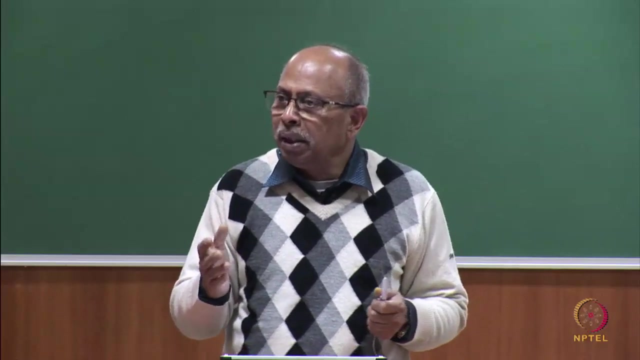 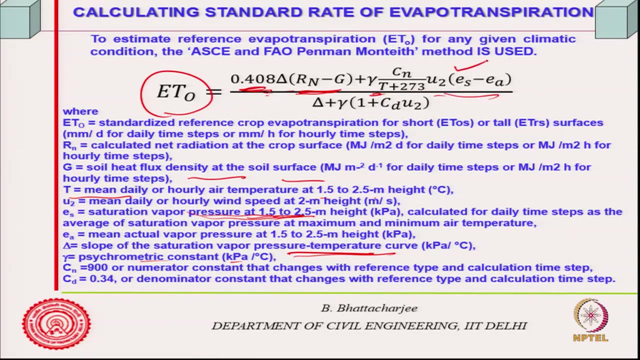 chart. absolute humidity, Relative humidity, dry bulb temperature or temperature. these are all related through psychrometric chart or, you know, at different degrees of saturation. what you call a different relative humidity slope of that curve is, you know, used. So here this is the saturation vapour pressure at 2 meter height. 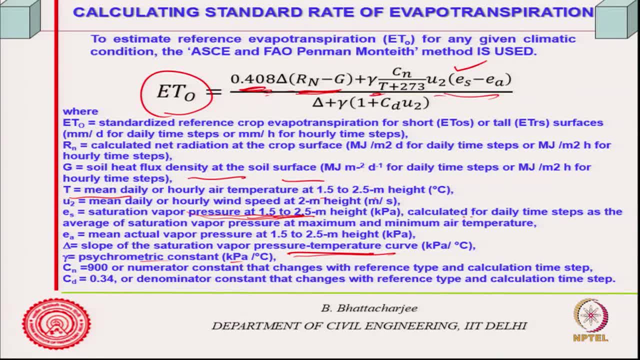 So you take from 1.5 to 2 meter height Calculated for daily timings, Time step, because if you are doing it for 24 hours, so you will do, you know, assuming that this is a kind of constant over a period of time: every hour or every half an hour or 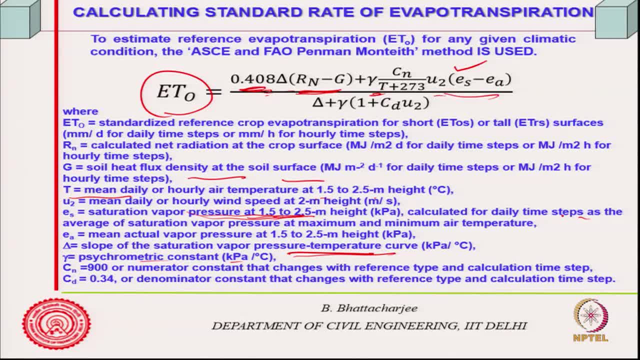 every 2 hours and it will depend upon you know it will calculate it for daily time. step Mean, actual vapour pressure. so this is the actual vapour pressure, this is the saturated vapour pressure at that height. ut is the velocity, because that causes the evaporation. 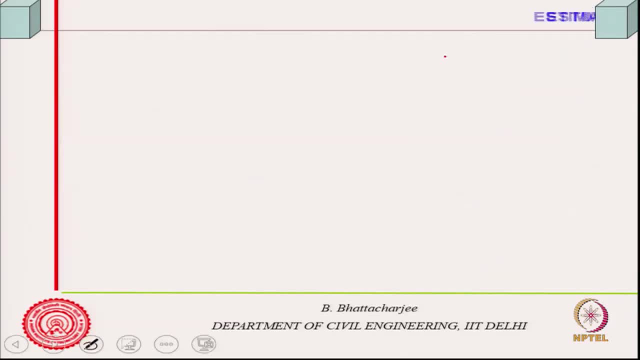 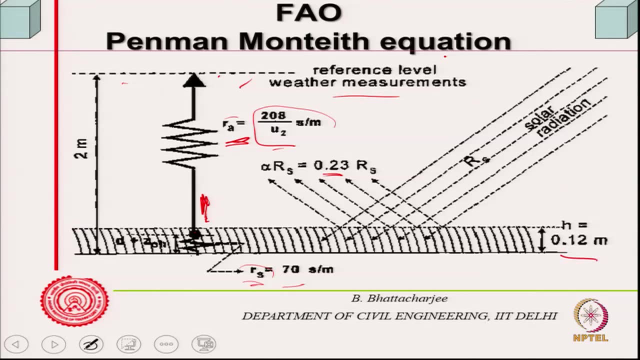 from the second stage. So, first stage, we saw, you know, this part- 408 Rn, etc. Deals with 408.. 408 Rn, etc. etc. deals with this situation. It deals with here, evaporation at this level, and this portion is the second part. 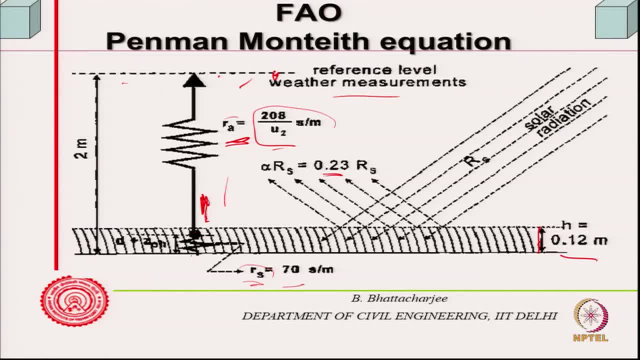 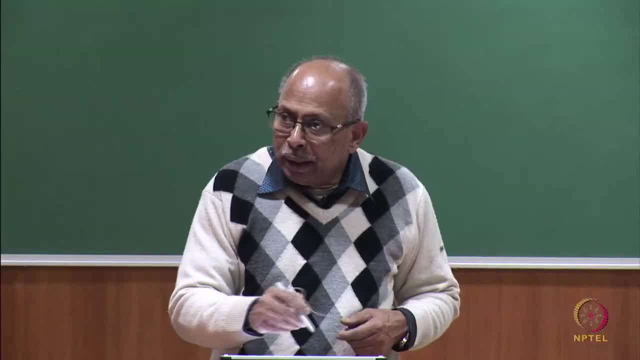 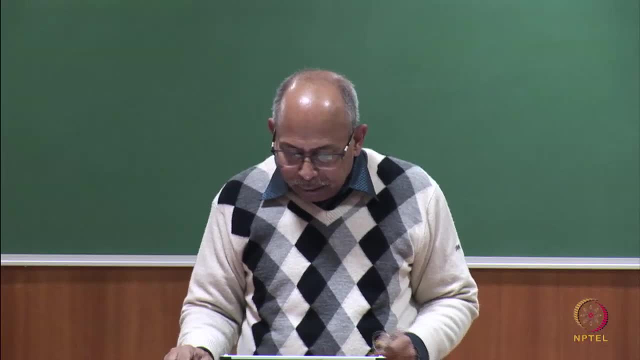 So the we are taking the saturation pressure here and the actual pressure there, So that difference will cause evaporation occurring at. you know, from here to there, evaporation occurring right. So that is the two part of this equation. That is the two part of the equation. 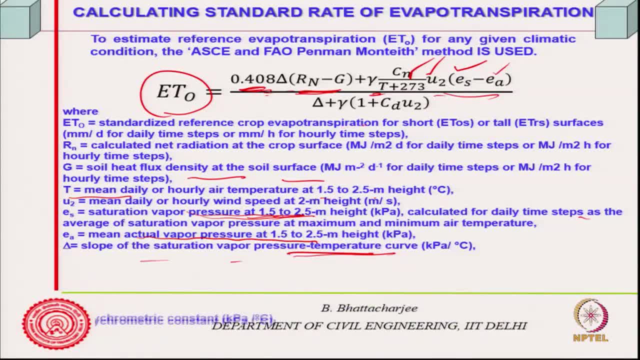 So this is a constant and this is another constant. Now this divided by the psychrometric constant and ratio of this two resistances, ratio of this two resistances. So you can see that this is the radiation falling in direct radiation. G is the soil heat flux, the amount of heat radiation going through the soil. 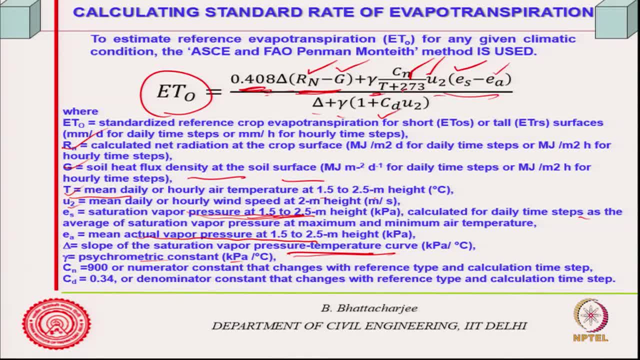 T is the mean temperature at 2 meter height. You know this is where it is coming. This is saturated vapour pressure at 2 meter. Partial vapour pressure at 1.5 to 2 meter height. This actual air pressure at partial vapour pressure at 1.5 to 2.5 meter height. 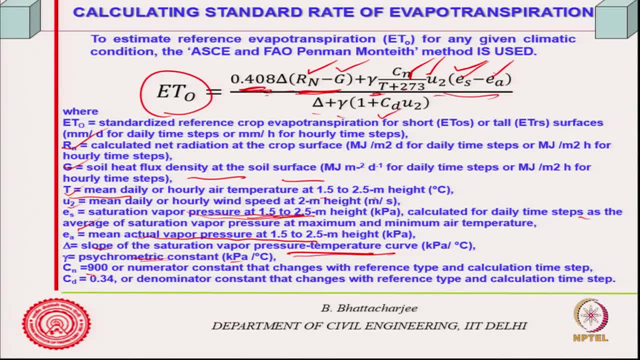 This slope of saturation line and this psychrometric constant. These are some constants depending upon time step you take for calculation, Because you will calculate at different times. assuming time step to be constant, during that period of time how much evaporation has occurred, So it will. 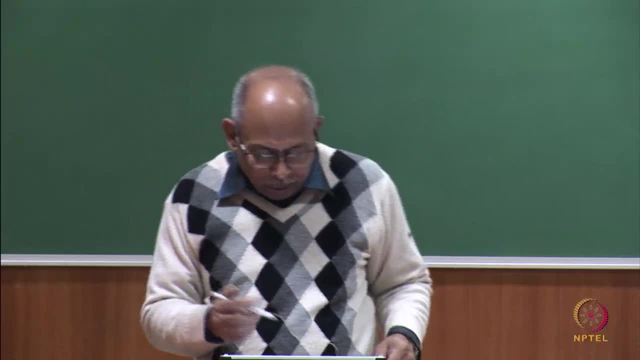 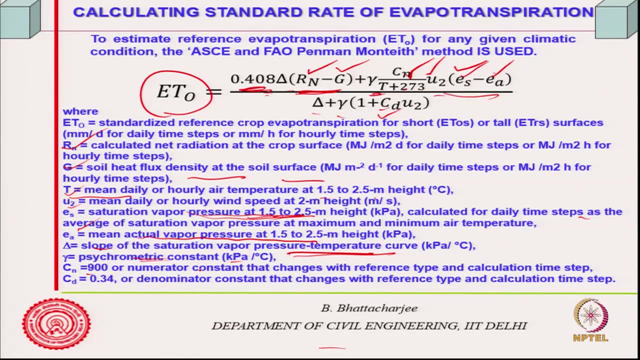 It will. It will happen for the whole day, Millimeter per day. that is what you will be interested in, And this values can be 34, ideal condition, or it can be some other values. So you see, one can find out the ET0. 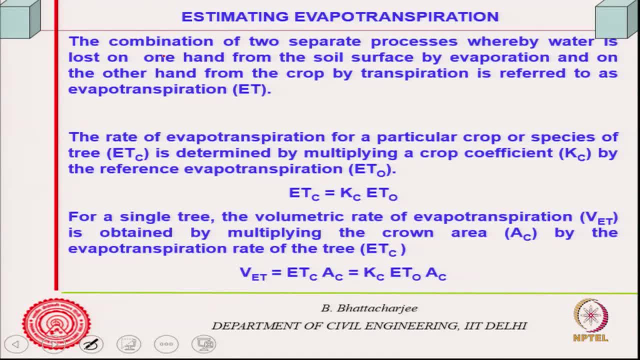 Then K values are available on table. K values are available on table. You know, K values are available on table. So this separate process whereby water is lost on one hand From the soil surface by evaporation and soil, the other hand, From the soil surface by evaporation, and on one hand, 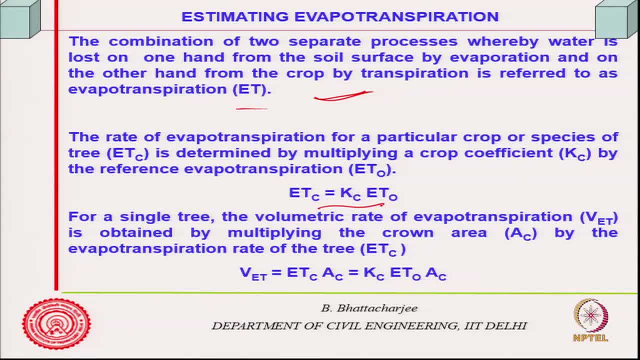 The girls you can read on the information you know. on the other hand, from the crop, by transpiration. that is what it is and this Kc. So the Kc value is, we know for different types of crop or plants, for assuming the plant, we 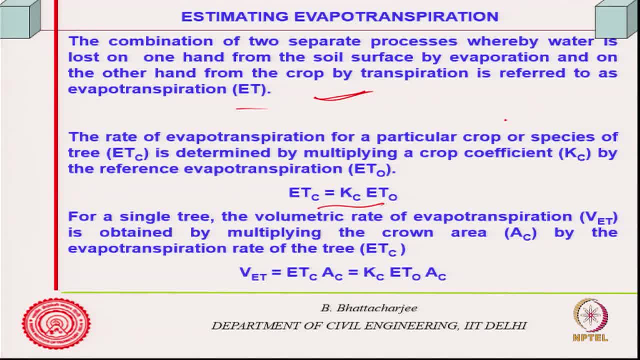 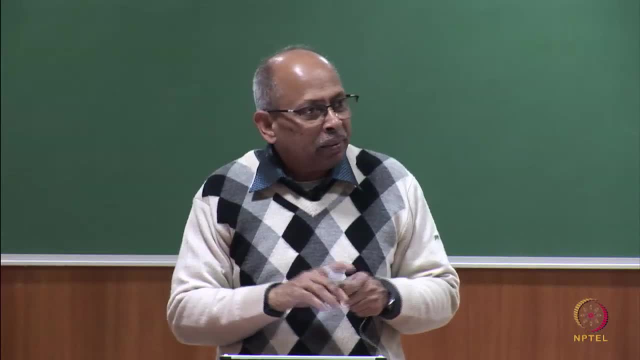 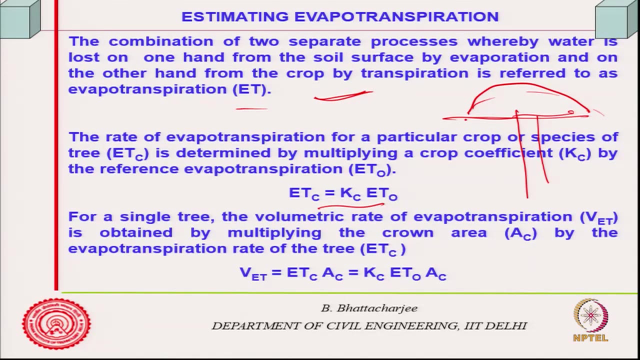 can assume our plant, supposing it is tree, a hemispherical surface approximately, because tree leaves generally form that is kind of an umbrella shape thing. So you can approximate this to a, say, 5 meter radius, 5 meter diameter or 10 meter diameter. 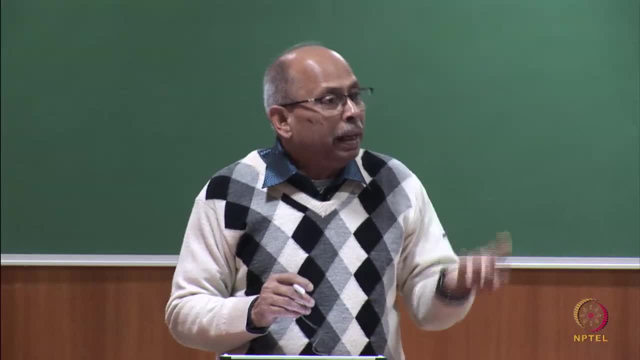 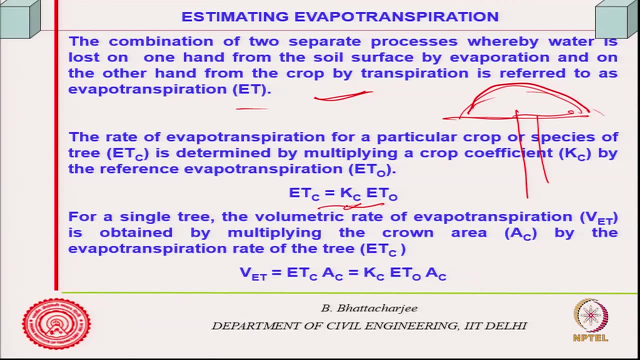 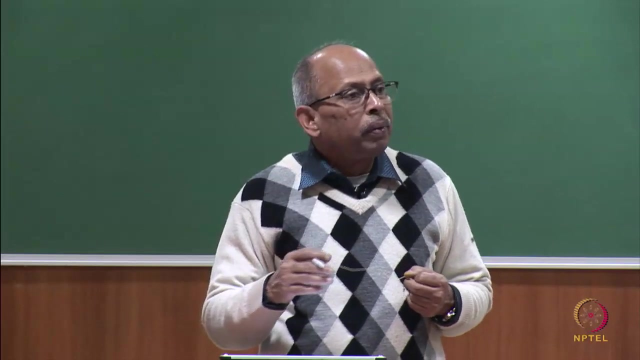 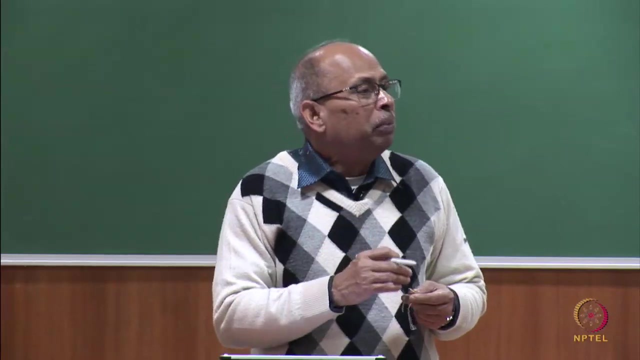 etc. etc. and for the given type of plants you have not really crop- the multiplying factor will vary, and thus whole list is available. for different types of plants, for example, I mean for trees- Supposing you want to convert it into Trees of the kind of, you know, like banyan tree- the values are available. so these values, 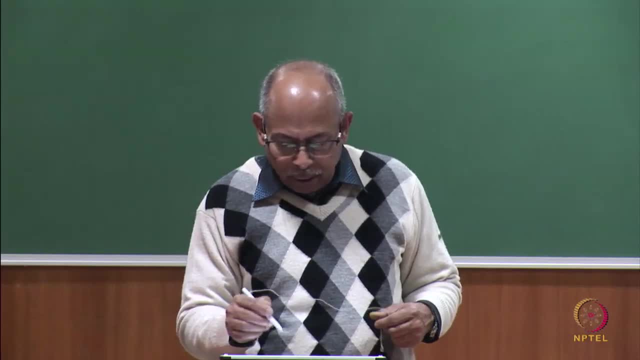 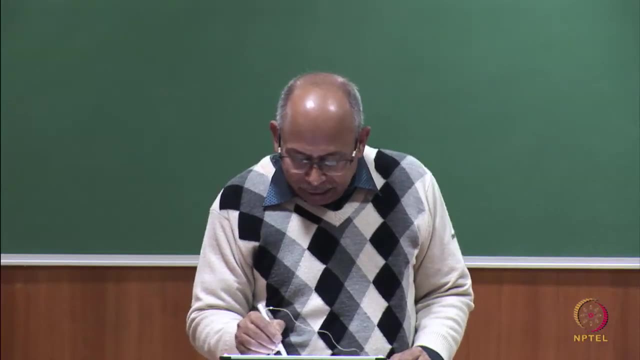 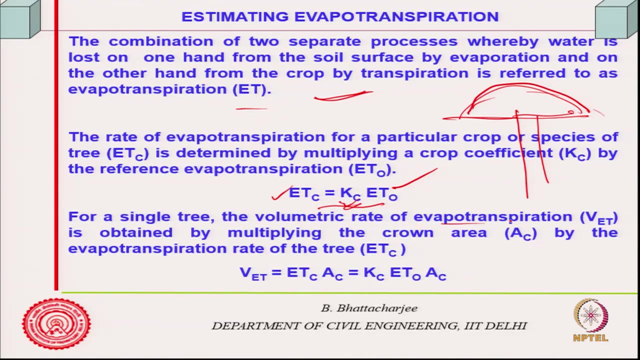 people have actually obtained the botanical. you know people with botanical background and things like that, or agricultural background they have. so this you can multiply, standard one, you can calculate out and this is what you find out. Now, for a single tree, the volume of creative evaporation is obtained by multiplying the. 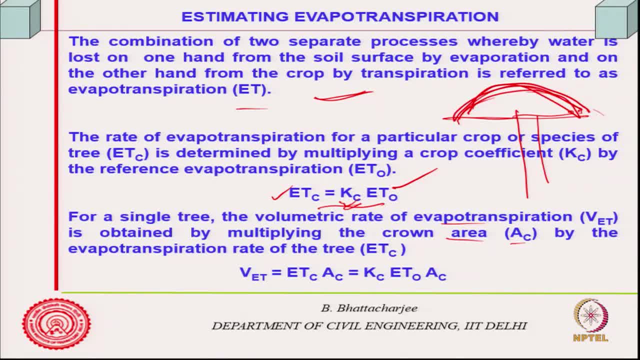 crown area. So this is the crown area. the crown area will be simply Pi D square by 2, because we assume it to be hemispherical, right, hemispherical right. okay, it is Pi D square by 4, Pi R square, so Pi D square, so Pi D square by 2. that is what it would be. so crown area by the you. 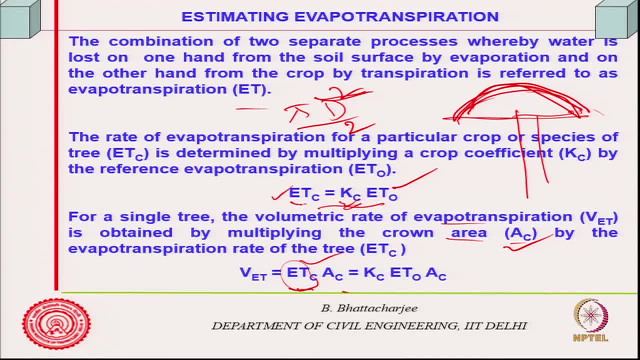 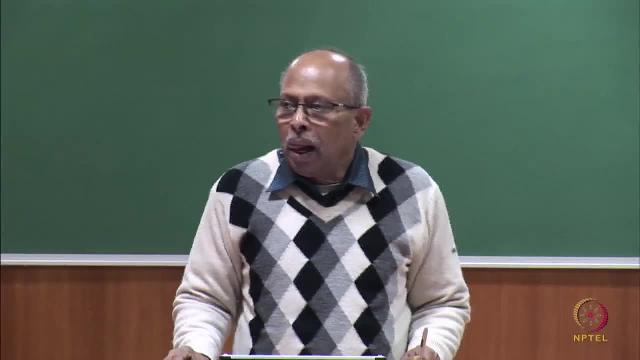 know. So you get E, T, C standardized value: E T, C, E T C. multiplying by crop factor and moisture factor and all those this multiplies the volume of, you can actually find out K, C, A, T, C, A, C, right? So for example, the example that K C we will take later on Humein's tomb, let us say where. 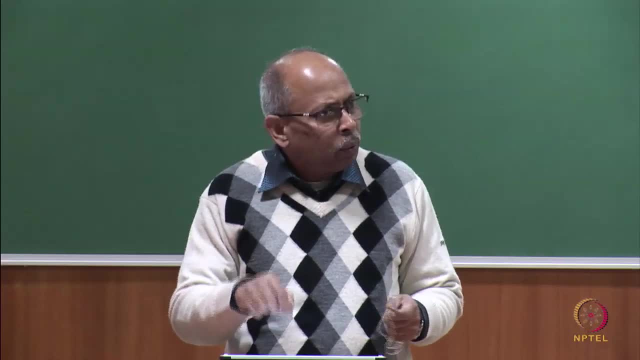 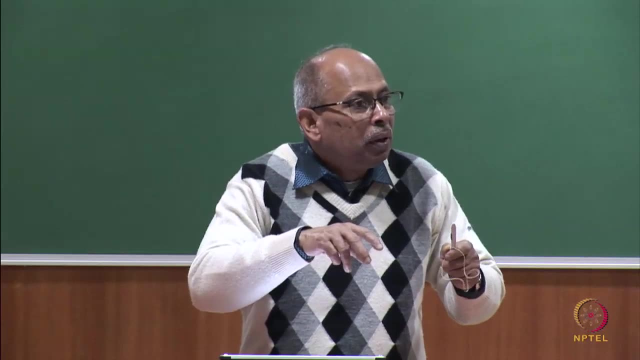 one could count the number of trees. if you see that I have some Google photograph of the same, I will show you. the actual tomb is there. surrounding that there are number of trees of different sizes. Some of them are very large, Some of them are very small. 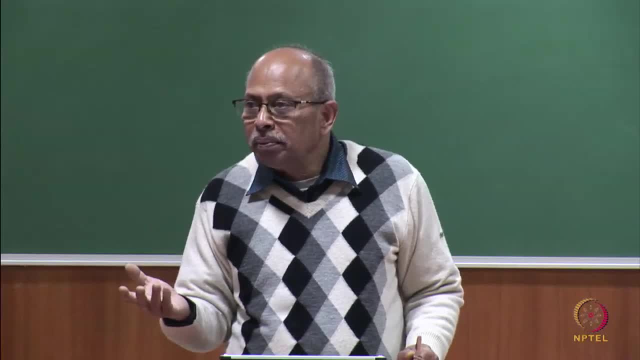 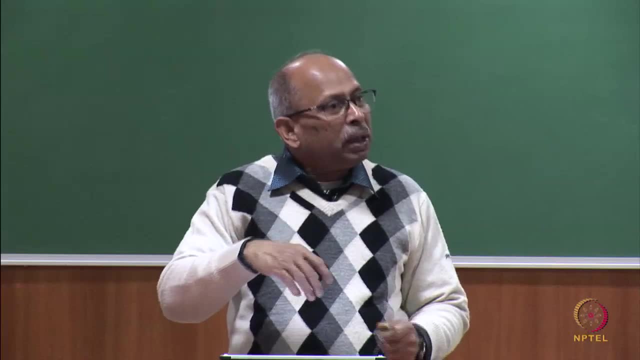 Some 5 meter, Some 10 meter, So one could count them. and once you have counted, counted them for the whole day. you want to find out how much is the moisture that will evaporate from the tree top, from the crown. So that is given by this formula. 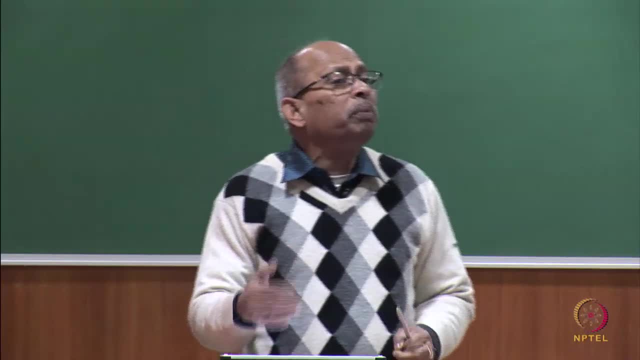 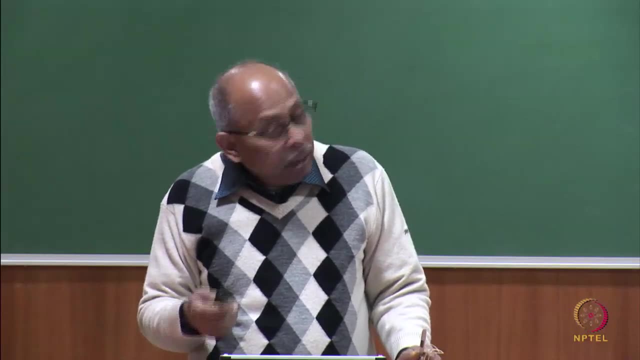 Now you cannot do. hand calculation may not be very easy. remembering the formula also may not be very easy. remembering the formula also may not be very easy, but you can write an excel sheet so easily you can actually calculate out. Now, once you have calculated that, what you have found out. 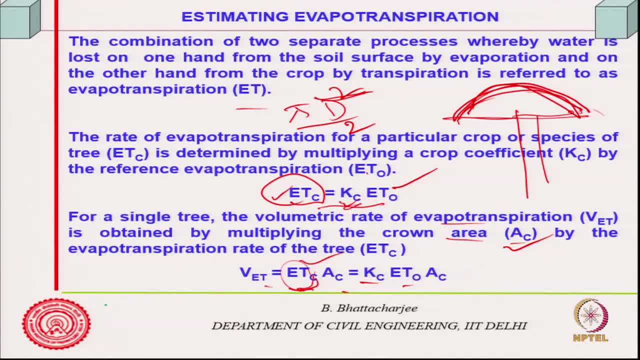 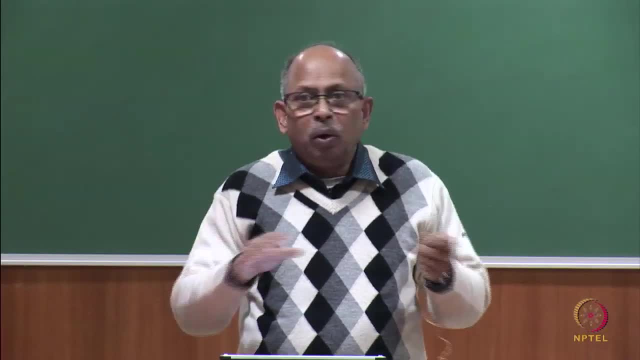 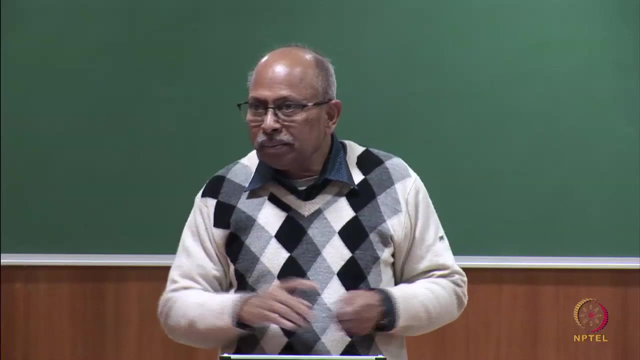 The evaporation that is occurring, evaporation that is evaporation that is occurring here. you know, evaporation that is occurring, actually evaporation that is occurring at this level. Now, this will not remain there. this will get distributed all over the space. So you have a kind of a space that you are concerned about. consider that total space. 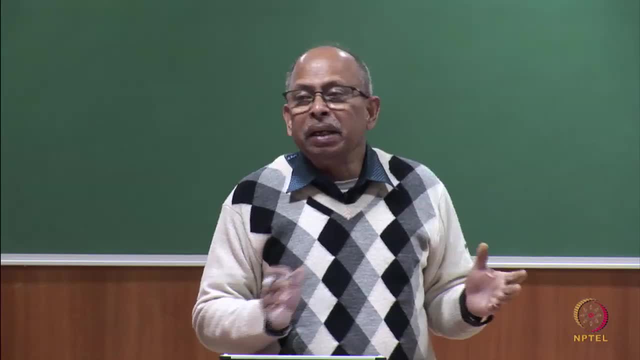 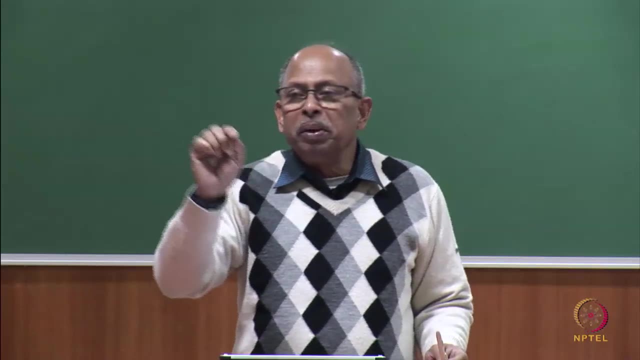 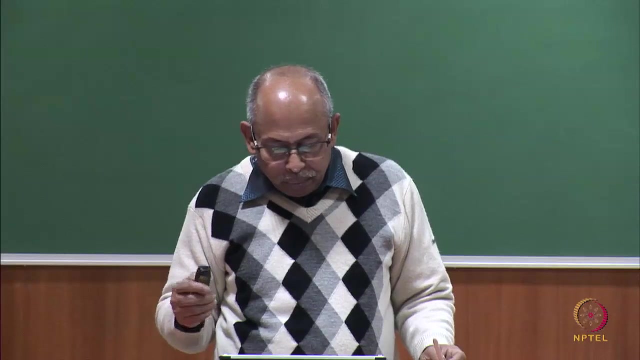 it will be a 3 dimensional space, could be a rectangular parallelepiped, Because there will be number of trees and then you want to find out what would be the relative humidity at every element in that area, right? So that is that you can do. 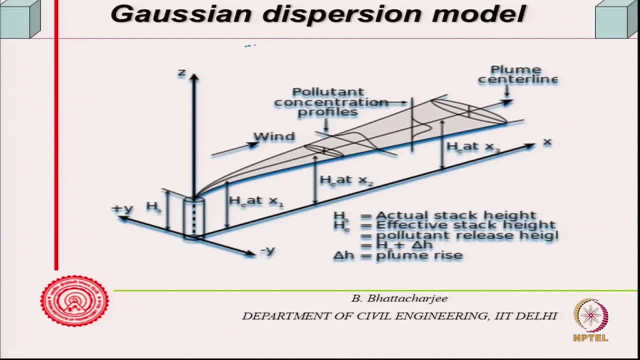 Now this can be done using what is called Gaussian dispersion model, which have people in air pollution use. you know, when they have a steady situation of a chimney, let us say vertical one, The pollutant or smoke moves along. it is assumed that it actually moves in a with circular. 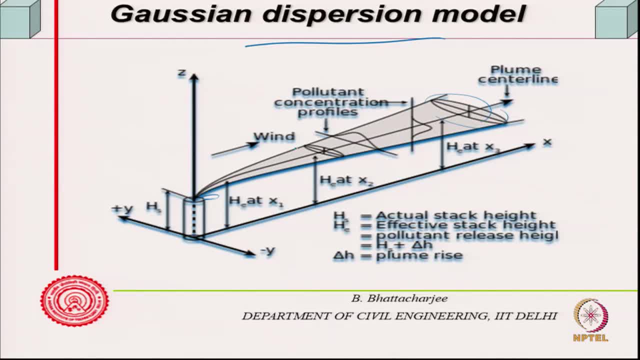 cross section. it expands and moves in a circular cross section. So if you look at the direction of movement, take a normal path, I mean normal direction- it will be circular cross section And you assume that in all both the direction it is normally distributed. The concentration is maximum at every element. 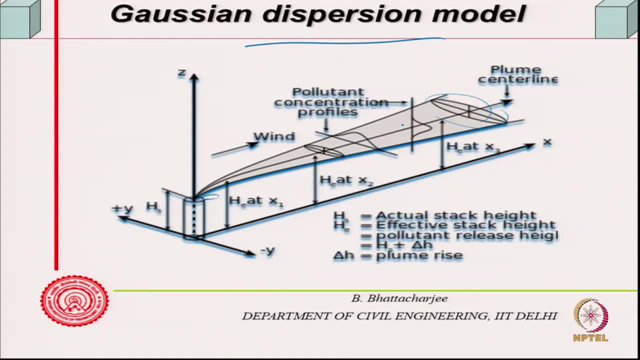 So if you look at the direction of movement- take a normal path- The concentration is maximum at the center and symmetrically distributed about the center, like Gaussian distribution. So this is Gaussian dispersion model. that is what it is. So pollutant concentration. So in our case this can be our tree with the height hs. this is x direction, this is z direction. 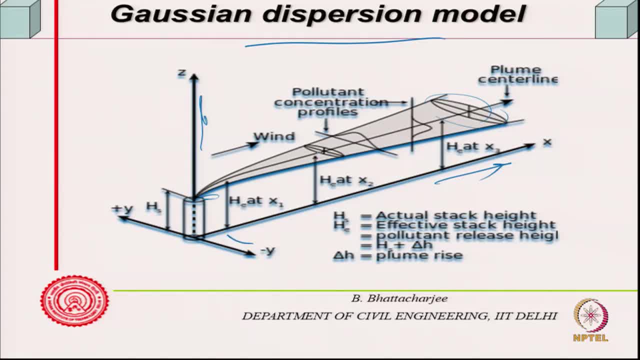 this is y direction, for you know, for a given tree, and therefore at a given distance, given height compared to this, Or given distance in x and y direction, using Gaussian dispersion model we can find out what will be the moisture content right For a 3 dimensional box kind of an area where this might be my tree height. there are number. 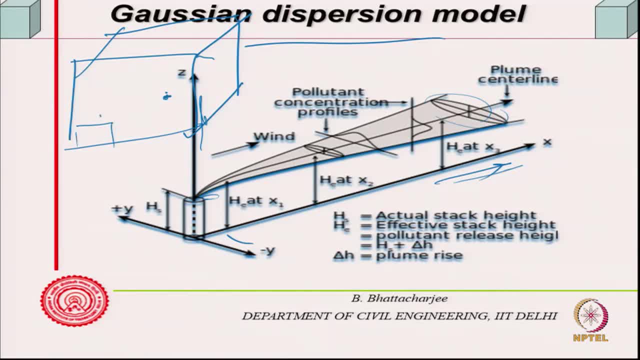 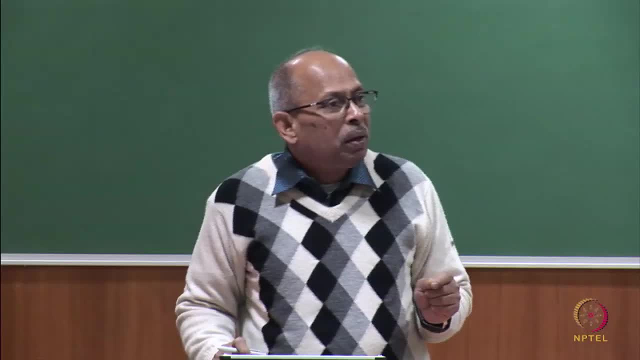 of trees and that I find out at any point. I can find out the moisture content from a single tree. I can sum up for all the trees to find out What is the. you know how much will be the dispersion of the moisture vapour from the. 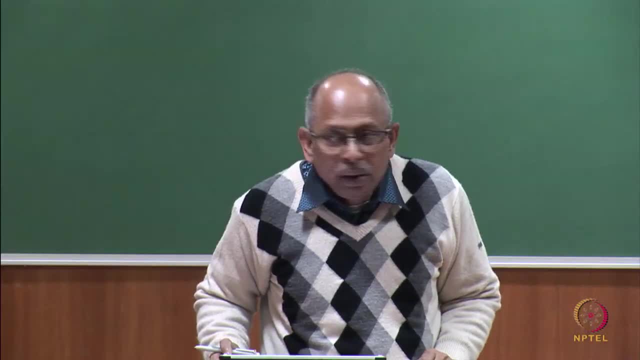 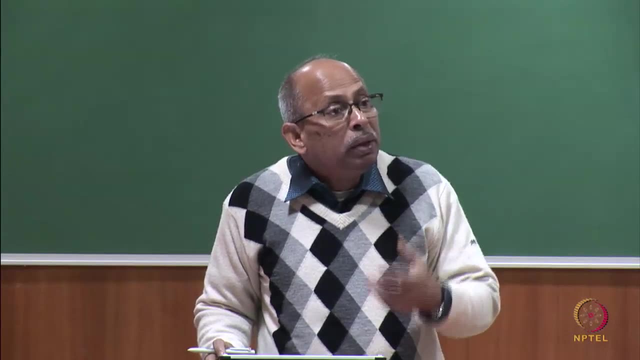 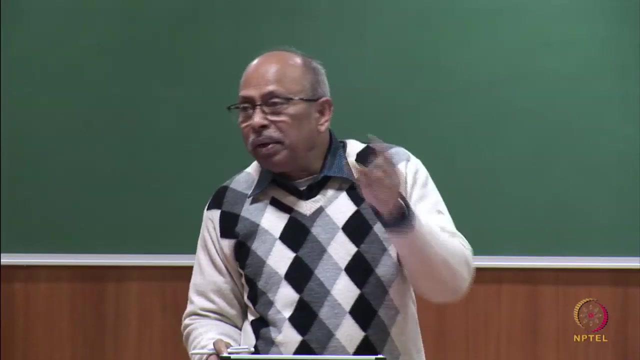 tree to that, from all the trees I can find out. Now, this moisture vapour actually, you know, would reduce down the temperature because it would, it would have taken the latent heat of evaporation. So on an average basis, total temperature reduction we can find out. 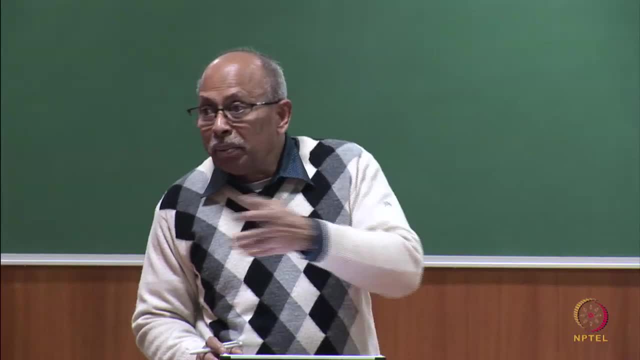 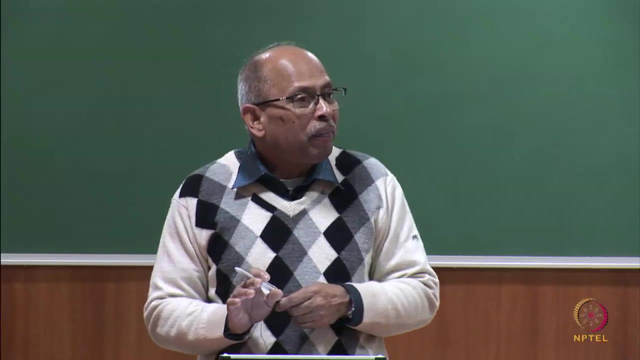 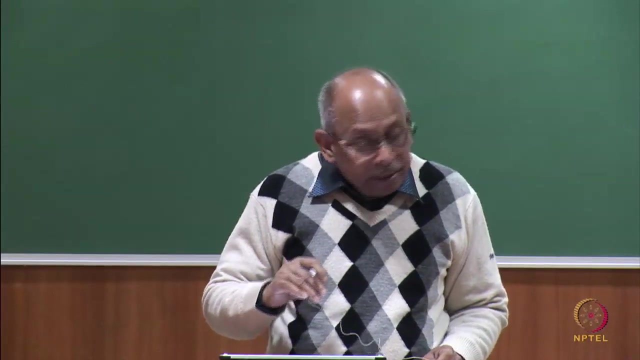 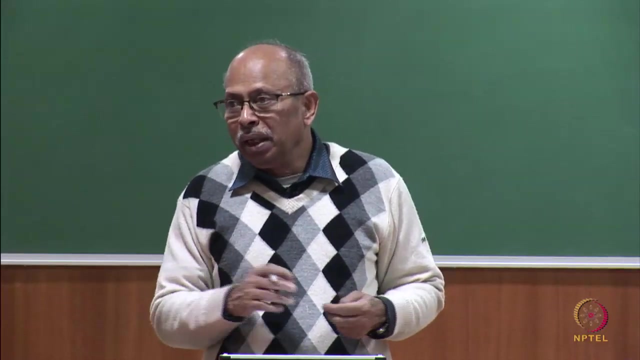 Because the amount of moisture that is evaporated, sum total of all of them divided by latent heat of evaporation, will be the average temperature change in the whole space, right. Average temperature change in the whole space and the moisture that is added actually change the relative humidity will change the relative humidity, right. 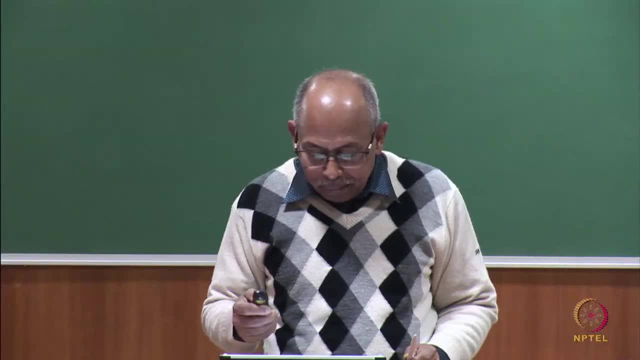 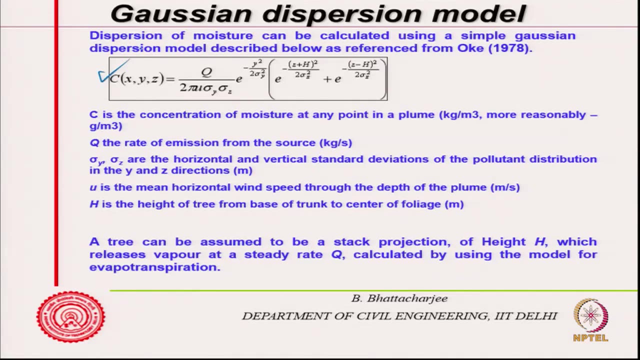 So that is what it is. So Gaussian plume model is applied And the formula is something like this: Concentration, or in our case it will be mass of the moisture per unit volume at any point XYZ in any point in the 3 dimensional box, is given by Q, is the rate of emission from. 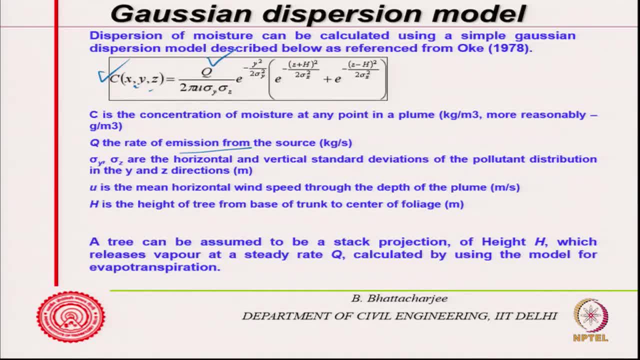 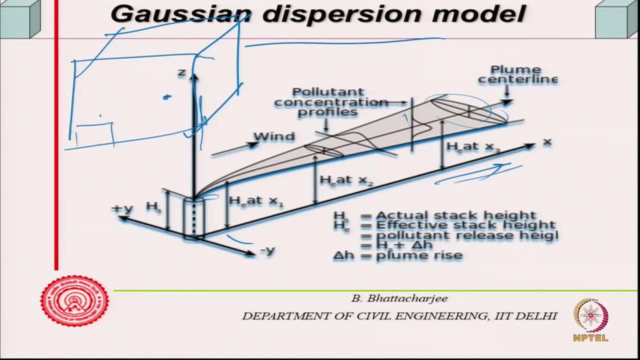 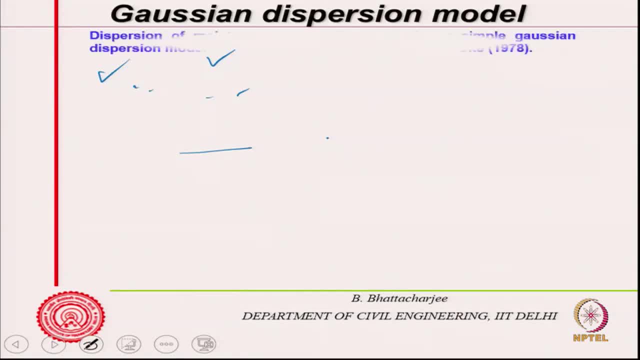 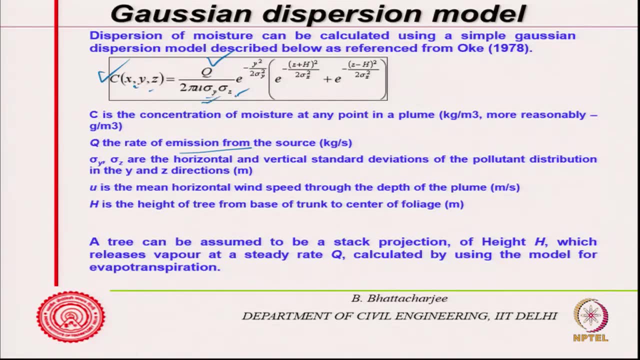 X and Y direction. So the spreads, these values are actually available. Values are available for different types of pollutants, how they will spread. actually, these are available. So sigma X, sigma Z, U is the air velocity mean horizontal speed to the depth of the plume, horizontal air speed. 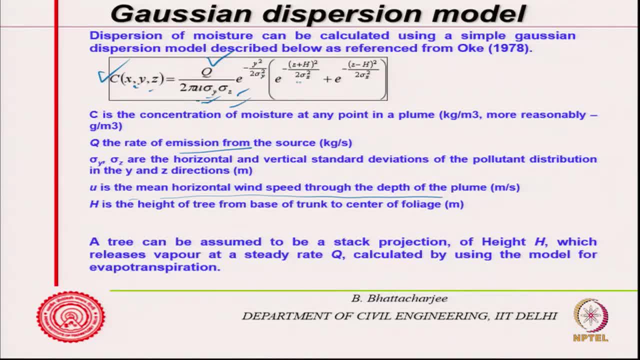 right, given a direction of the wind, and this is Z is the height in Z direction. H is the height of the tree from base to trunk, base of trunk to the center of the foliage. that means half of the crown, you know, center of the foliage. 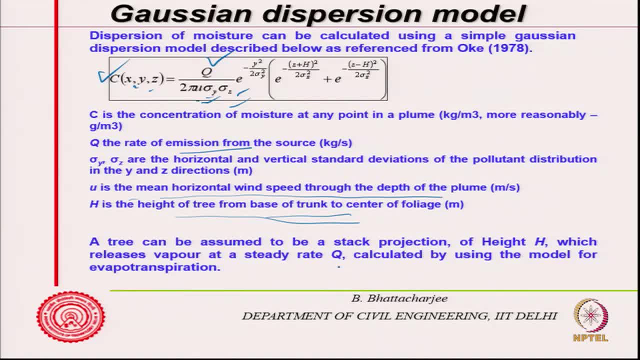 Okay, So you can assume the tree to be a stack projection of height H, which increases vapor at a steady rate. So this is valid for steady state situation, constantly evaporating at the same rate. moisture is constantly evaporating at the same rate, right? So this is valid for steady state situation, which releases vapor at a steady rate calculated.